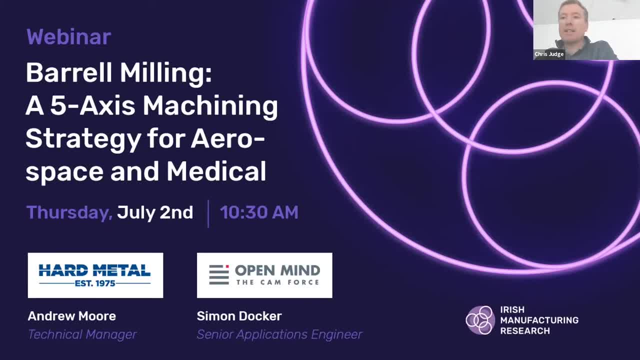 to demonstrate this technology, which uses different types of toolpaths and tooling. We've invited two IMR partners to discuss this with us: Andy Moore from Hard Metal, representing Moogie Franklin and Nisgaard, and Simon Docker of HyperMill, with us this morning. 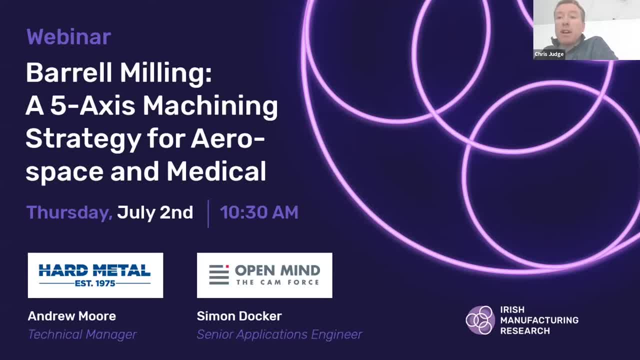 Both of these guys are experts in their field, and the Moogie Franklin and HyperMill companies were heavily involved in developing this technology. So, Andy, off to you, please, is. Thank you very much, Chris. Good morning everybody. As Chris indicated there, I'm Andy. 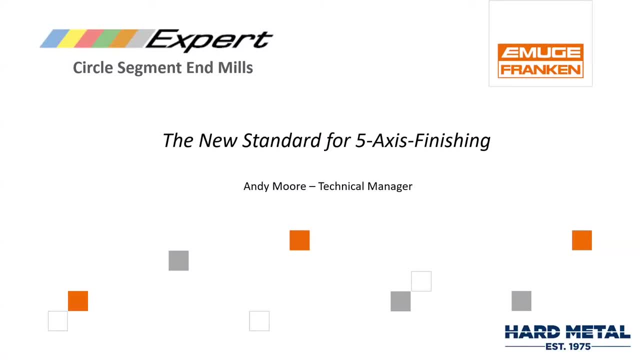 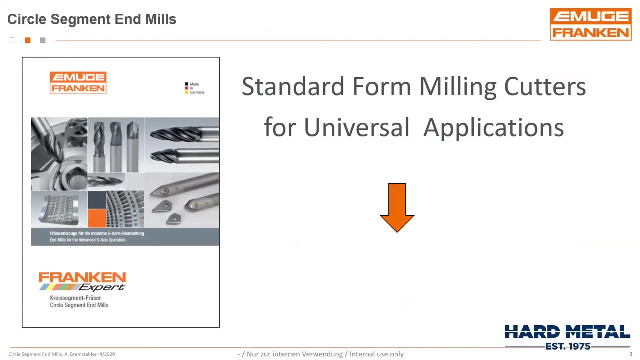 Moore, Technical Manager from Hard Metal. and today I'm going to introduce you to two companies, both ISCAR and Imugi Franken, who have been involved heavily in developing the 5-axis milling strategies using the concept of barrel milling. Imugi Franken has a full range of standard milling cutters, but 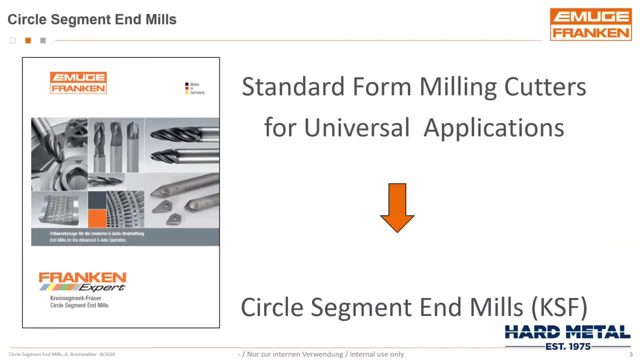 today I'm going to be talking about what they would call as circle segmented end mills. Circle segmented end mills have the possibility to reduce cycle times by up to 90%. How we can do that is because, when we look at today's technology for producing, 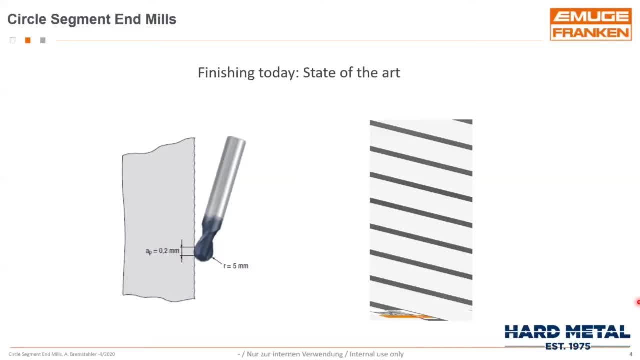 thin walled surfaces, high walls, concave or convex surfaces. we have to scan using a traditional ball-nosed end mill and typically, if we looked at a five millimetre radius or a 10 millimetre diameter ball-nosed end mill, we would have to take down steps of 0.2 of a millimetre. 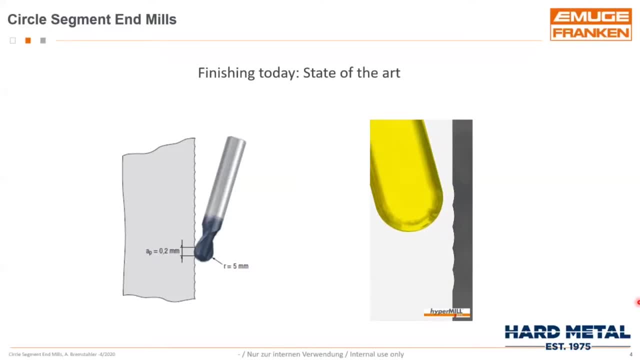 in order to be able to do that. So we have to take down steps of 0.2 of a millimetre in order to achieve a high surface quality. So we're trying to achieve a small cusp height between the two steps, and this is where we have to take small axial depths of cut, and this can be very time. 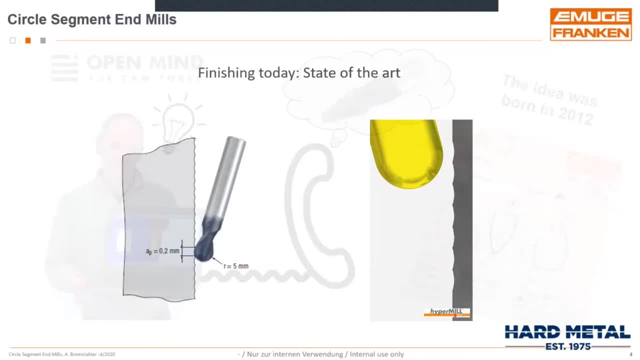 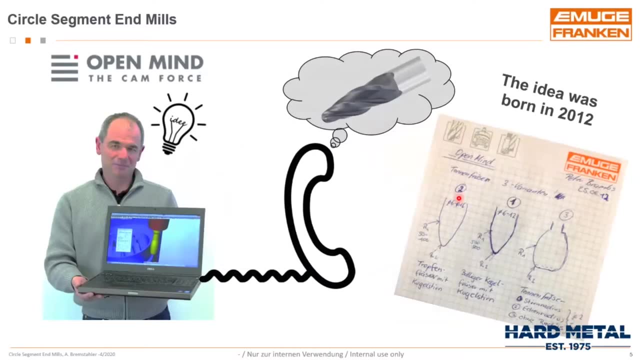 consuming in order to achieve a high surface finish. Back in 2012, Imugi Franken and OpenMind got together and tried to think how they could solve this problem of reducing the cycle time dramatically And on a sketch of paper, they basically came up with the concept of circle segmented tools. 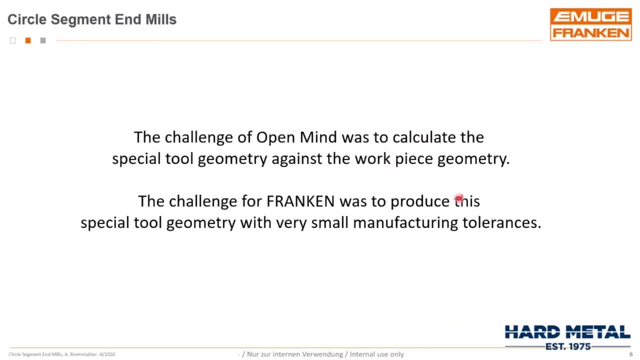 So how does the system work? Firstly, it was a challenge for both OpenMind and Franken together to find a geometry that would work against the work piece and for Franken to produce a tool geometry with very high manufacturing tolerances. So it was very much a partnership. 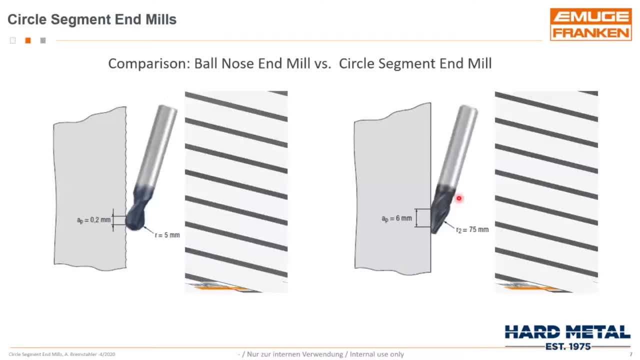 between the two companies to try and develop this technology. So again, just to reiterate, when we look on the left hand side, we see the traditional method of producing a thin water or a concave or a convex surface: small stepdowns, small cusp heights in order to improve the surface quality. Where you look now, 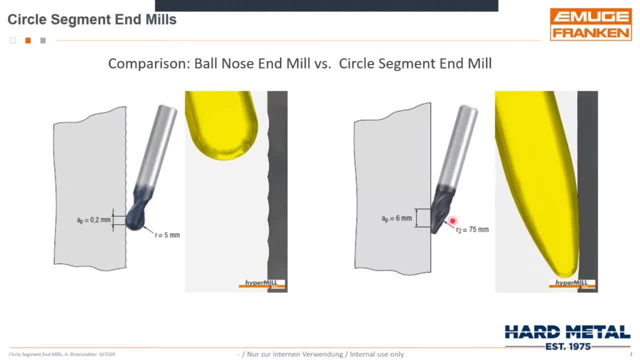 as to the right hand side, you see a very different shape tool where we have a large radius- R2 of 75 millimetres. This then enables us to take a much larger step down in the AP direction and create very small cusp heights between each wall. There's a lot of work that goes on in the AP system here. This has to be done, and if we put a lot of effort into it, we're going to learn something, and we're starting to learn something actually brilliant about the right hand side, you'll see a very different shape tool where we have a large radius- R2 of 75mm. This then enables us to take a much larger step down in the AP direction And create very small cusp heights between each wall. 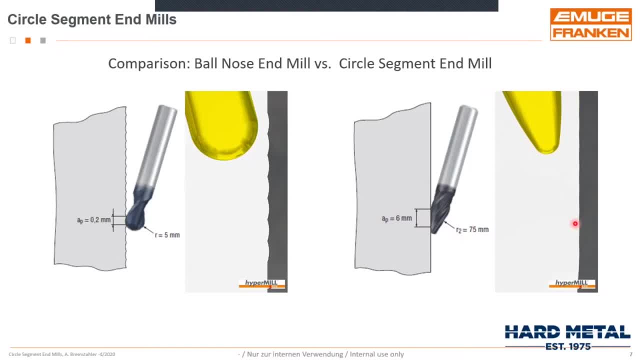 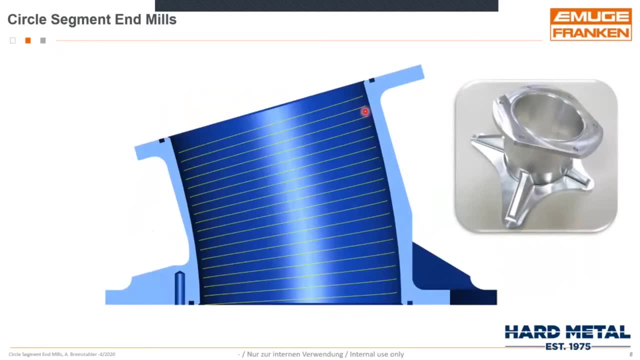 step down, creating a very high surface finish. So this is where the concept was born. If we put that into practice, if we look at a typical component here that we'd have to feature and produce this concave surface using a ball-nose, 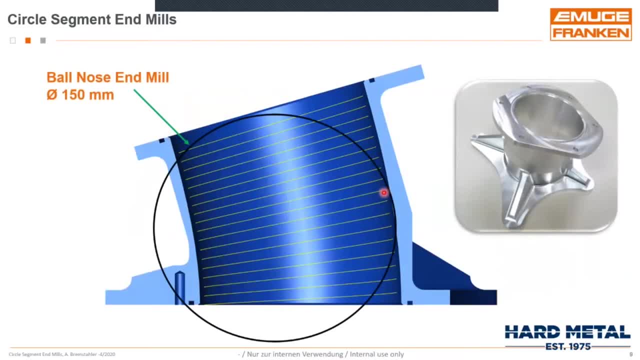 milling cutter. in order to achieve something with a 75mm radius, we'd need a ball-nose end mill of 150mm in diameter, which is totally impractical. So what we do? we take a tool, part section of a tool, and 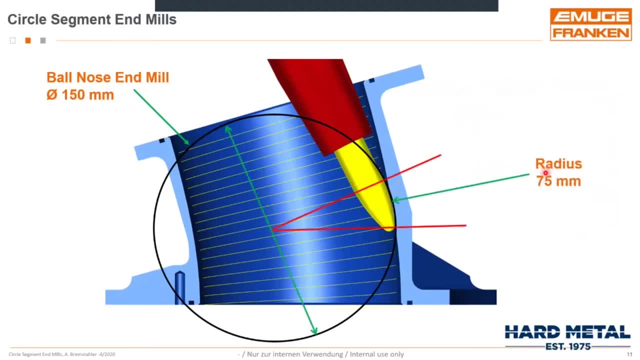 we create the radius of 75mm on a segment- hence the term circle segmented tools- And now we can produce that large step down, whereas conventionally we would have been using small step downs, And this is how we reduced the cycle time dramatically. Now there's four within the Franken range. 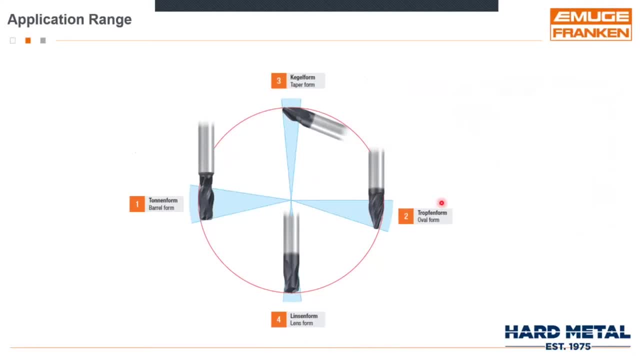 there are four types of circle segmented tools. Terminology barrel comes from this type of tool, where it is literally the shape of a barrel, But here we have restrictions in terms of the corner radius at the bottom and being able to get into tight corners. So here we have two options: either the oval, 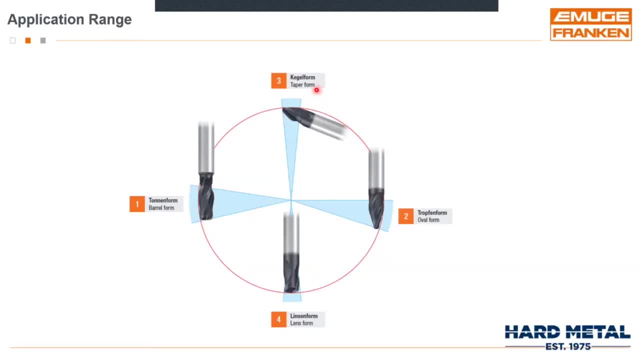 form or the taper form. Both function exactly the same but have greater radiuses depending on the two. But also both have a small conical radius at the end of the tool, which enables us to get right into the double fillet radius between the perpendicular wall and the horizontal. 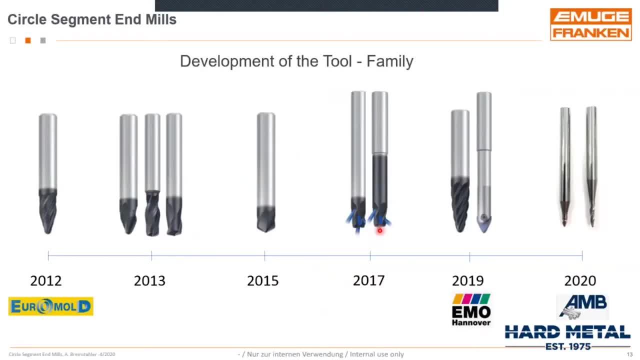 wall. So to summarize the range, and it was developed to say back in 2012.. The range expanded in 2013 to include two versions of the traditional taper and the taper tool and then in 2015 and 2013, they developed the lens type cutter. 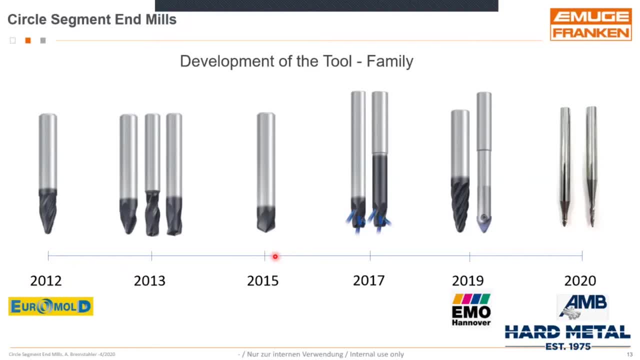 The lens cutter would be predominantly used for scanning flat surfaces or the bottom of pockets. 2017, a further expansion included basically tools for machining turbine blades and the like, So these were specially developed with special geometries and through-cooler capability. In 2019, they extended the range again with multi-flute type tools and even an indexable system. 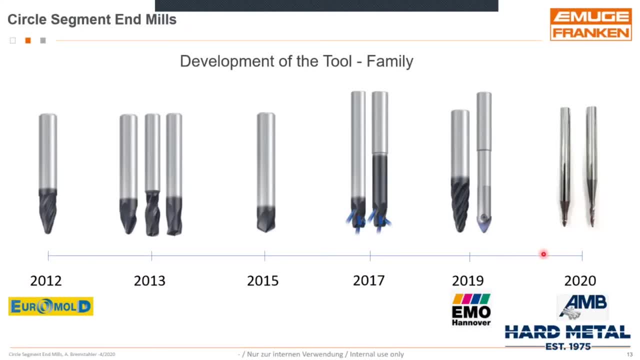 In 2020, the plan is to introduce micro-circle segmented tools or barrel tools, and that will be phased in over the course of the year. They were to be introduced in A and B but unfortunately, as we all know, all of those sort of shows have been cancelled. 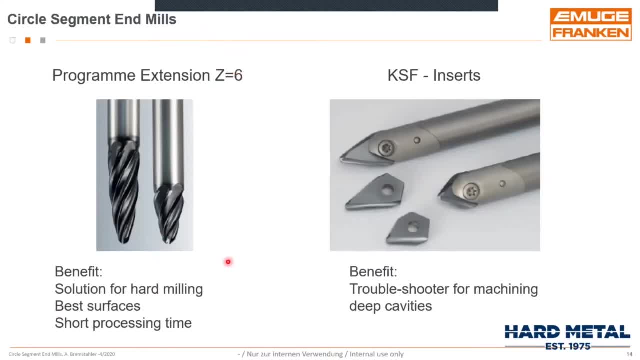 So just to summarise, multi-flute options: up to seven, up to six teeth, for both the taper form. These are used mainly on hard materials where we're taking small radial depths of cut. The new innovation of indexable systems gives us the flexibility to reach deep cavities. 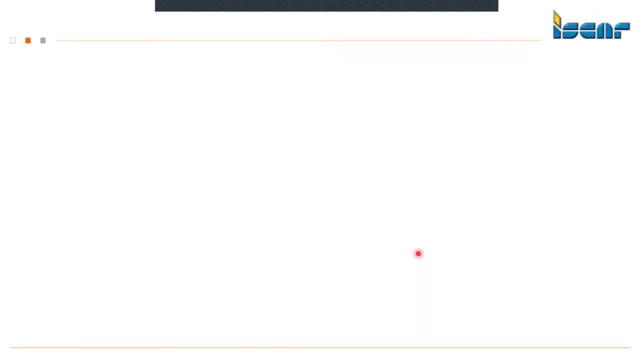 As a supplier of both Imugi Franklin and hard metal, being a supplier of also Iscar Iscar. Iscar has developed its range of circle segmented or barrel mill type tools, which gives us the possibility to work within the medical industry because of our experience with machining the lots of cobalt, chromes and titaniums. 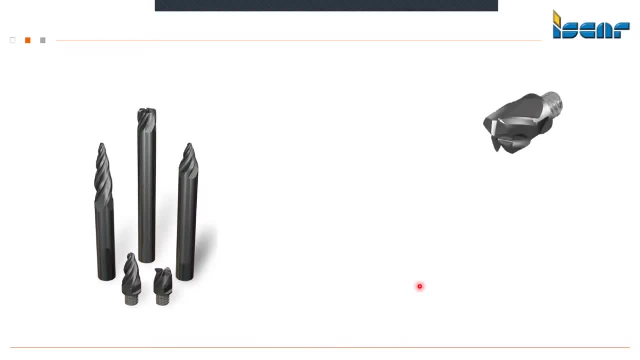 What Iscar have done is quite interesting in the fact that they've introduced the multi-master version, which gives us the possibility to use indexable heads in both the lens type, the tapered form type, as well as having the traditional solid carbide end mills. 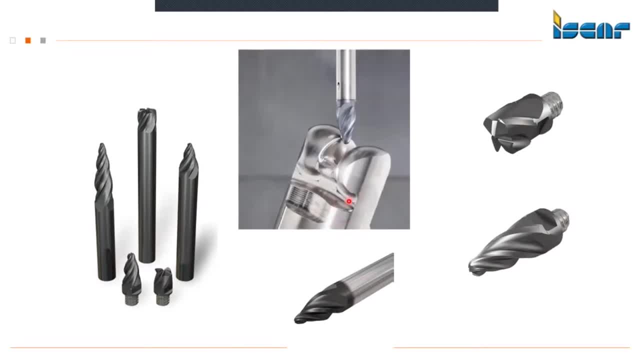 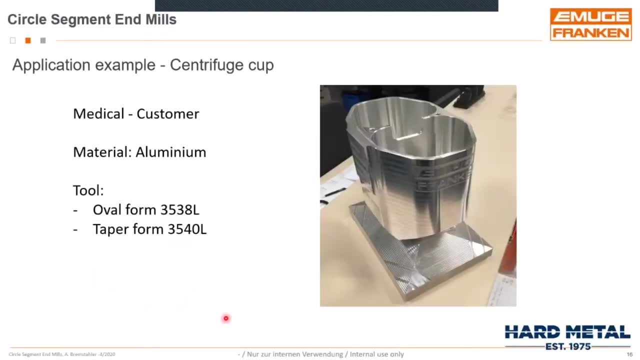 And, as I say, given our experience within the medical industry, we are actually looking at developing tools specifically for producing the lots of the femoral knee. I'm just going to show you just a couple of videos before I move over to Simon. And this is just to show you the tools in action. 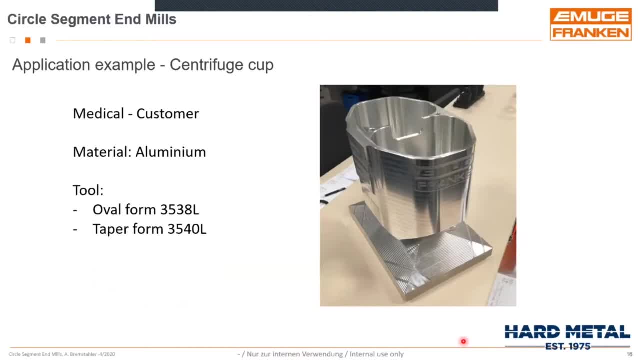 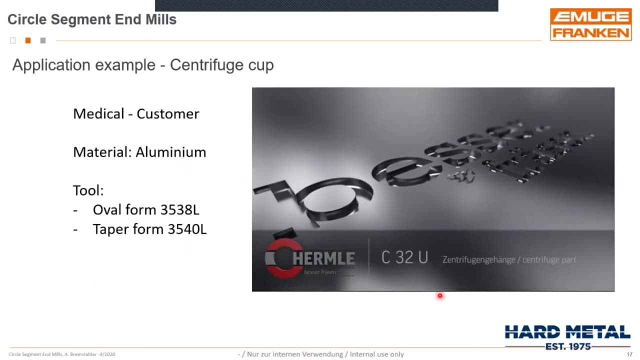 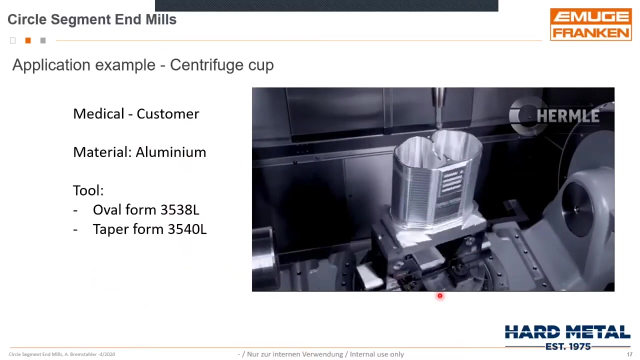 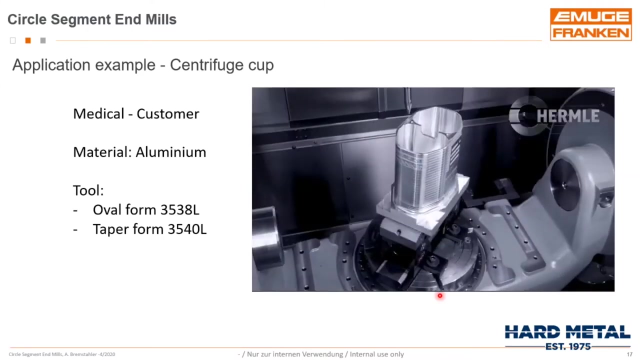 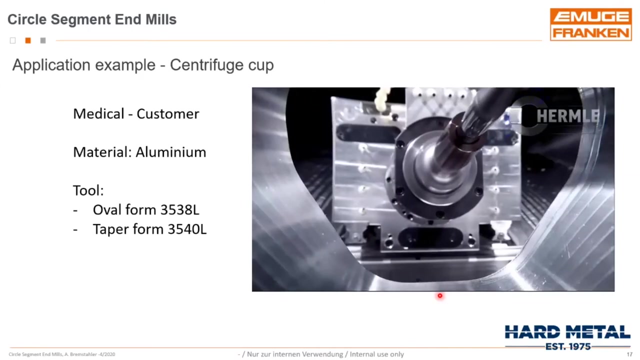 And this is an example of an aerospace type component- sorry, medical- a medical component made from aluminium using two types of the form cutters: the oval form and the taper form. I'll just run you the video now, But there's no problem with it. 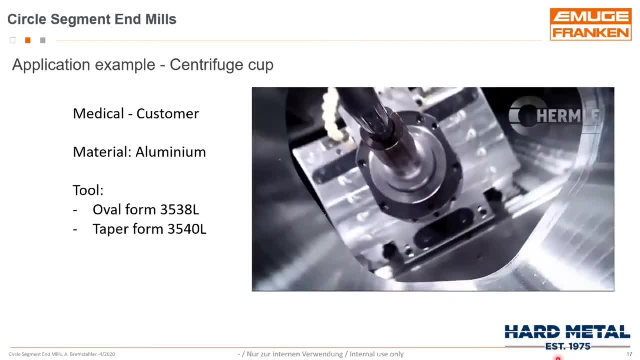 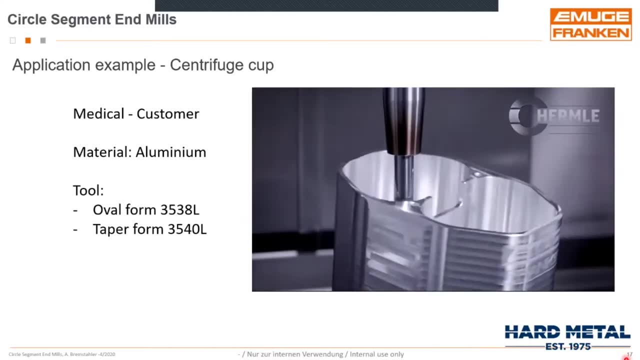 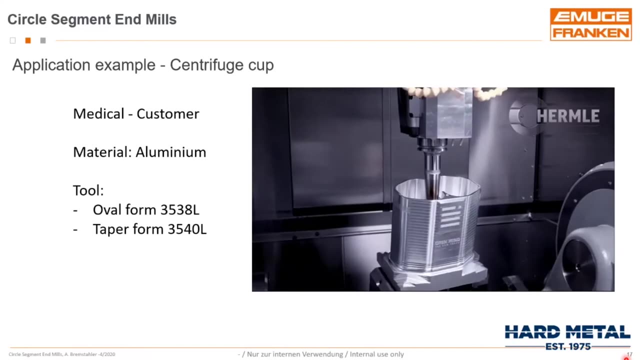 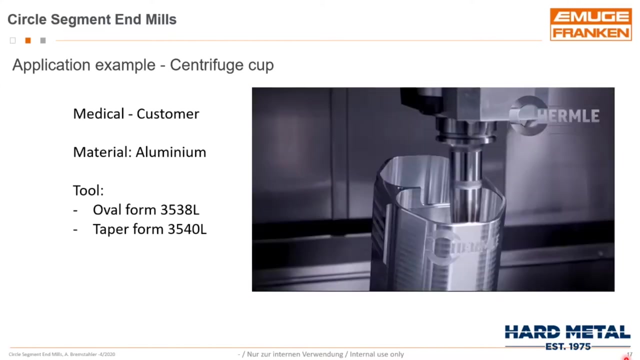 If I just go in and press the button and then press the button and then press down on the red dot and then press the button, then the I'll just press the button, And so theILL can do a little bit of it too. 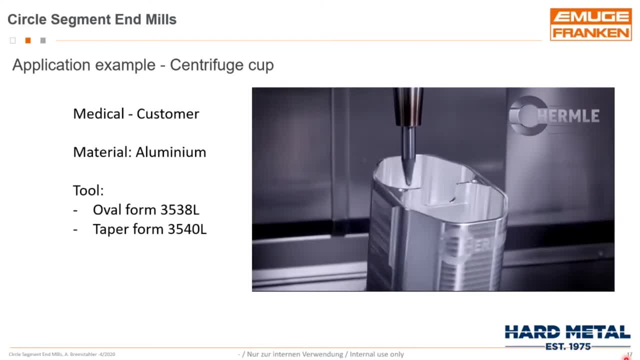 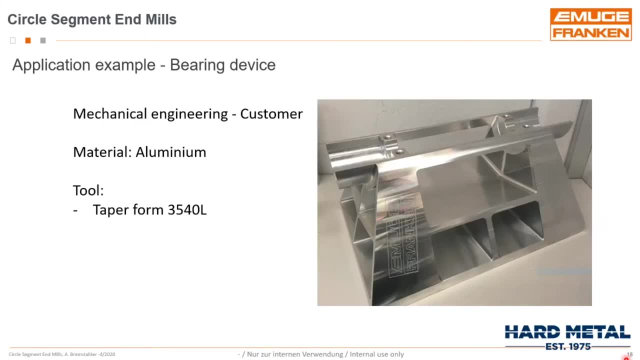 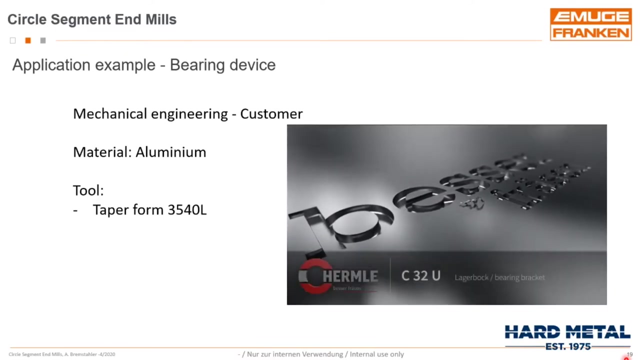 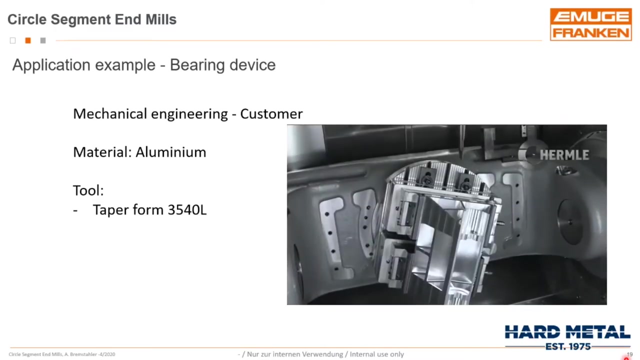 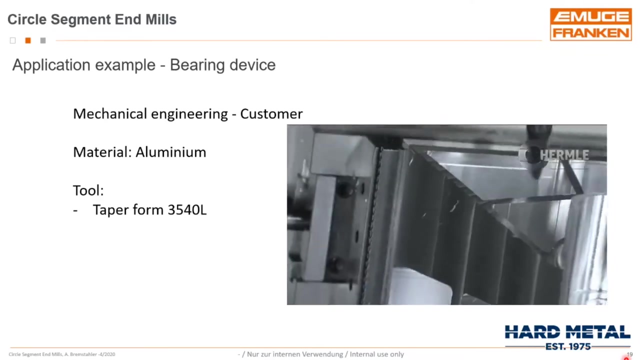 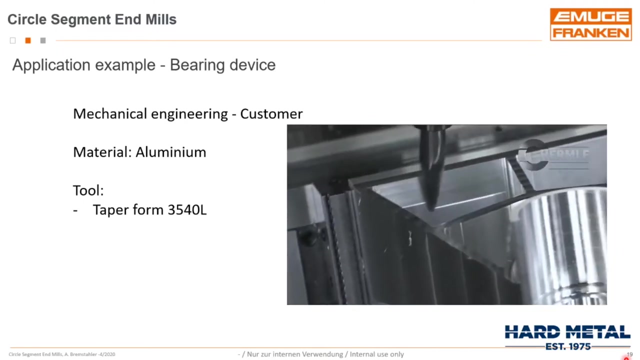 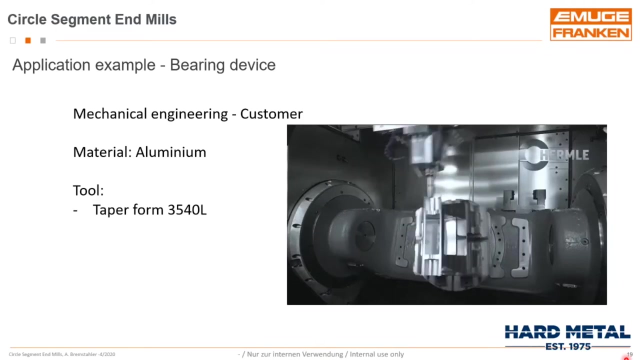 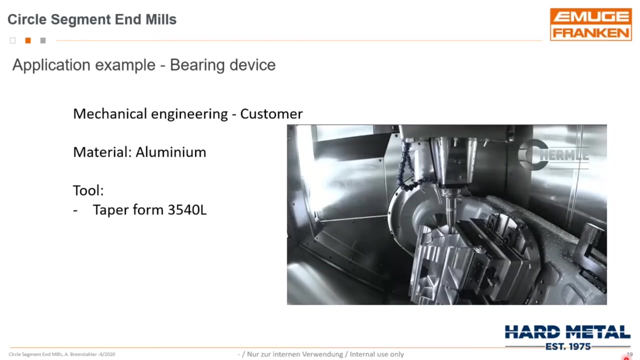 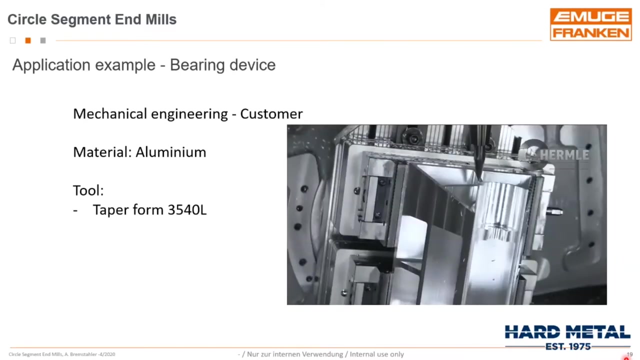 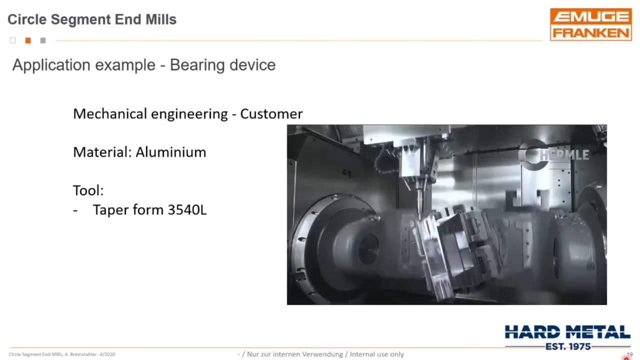 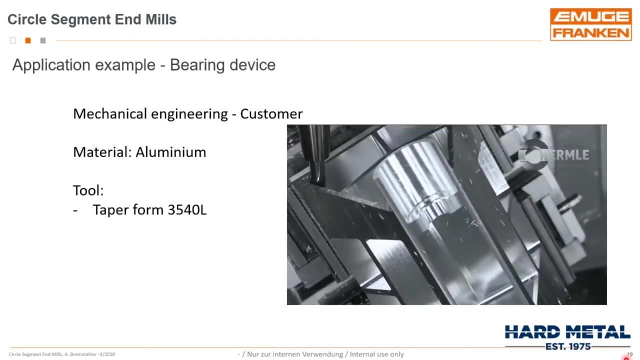 okay, just moving on. that's the next video, the rest of which basically just face machining. so this is another example. this is using the tapered form tool, again an aluminium component, mechanical engineering. it's just showing it all again in a different, different, slightly application area. you Thank you. 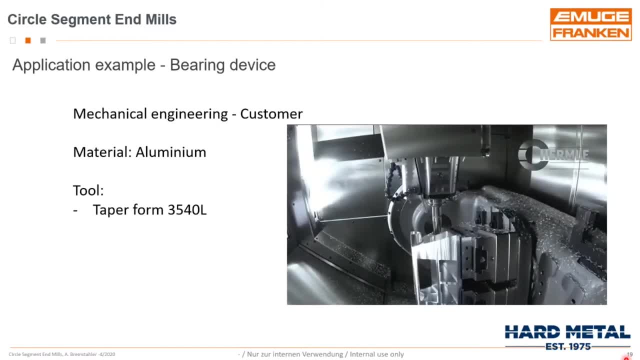 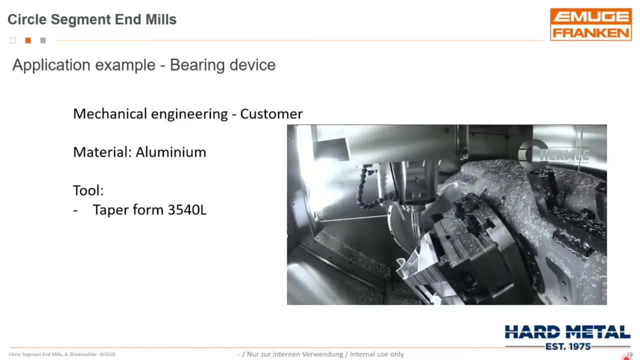 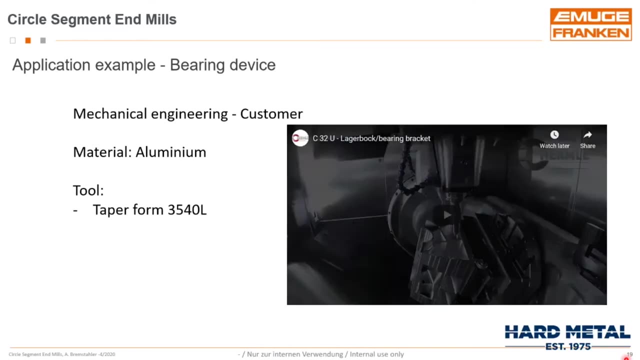 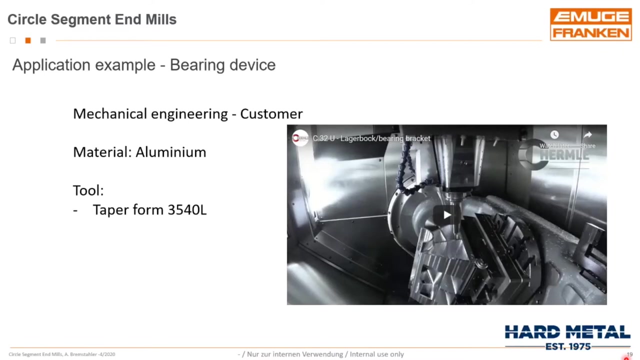 Okay, what I will just add before I hand over to Simon is that it's key to use the CAM package is vital in the success of using circle segmented tools or barrel mill type tools. So I'll now hand you over to Simon Docker from OpenMind. 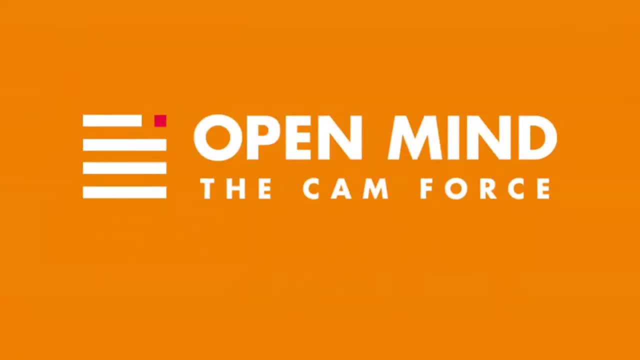 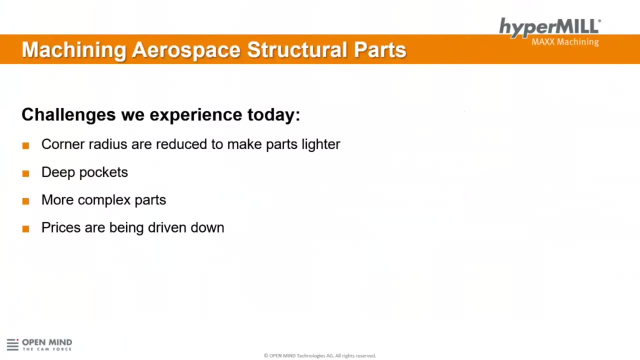 Okay, well, thank you, Andy, And and also thank you to the IMR for inviting me to join this webinar this morning, Much appreciated. So I'd like to focus on an aerospace structural part in the next few slides and some of the challenges we really that we experienced today. 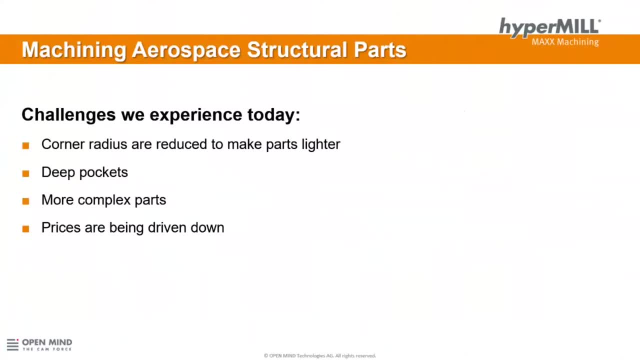 We've seen that the corner radius in pockets have been reduced to make parts lighter and I see some very deep pockets, And when you combine a small radius in the corner with a deep pocket is creates a machining challenge. parts are becoming more complex and, certainly during the current situation, prices have been driven down. So really, how can we be more efficient, more productive and reduce costs? 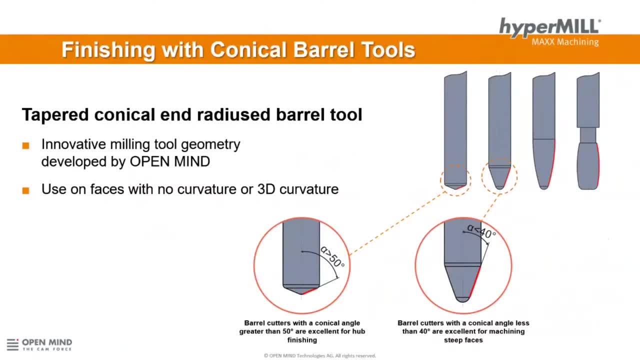 Now, as Andy has already touched on how we can achieve a faster cycle, we can achieve faster cycle times using a combination of conical barrel tools, or set circle segment tools, as they may be called. But let's look at how this is possible. 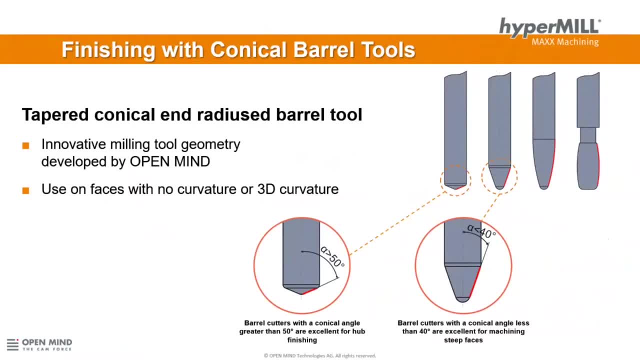 So what is the concept behind the design of a conical barrel tool? Well, as you can see, there is not only a long radius along the flute length of the tool, the tool is also tapered and ball nose. now, referring to this tool here, 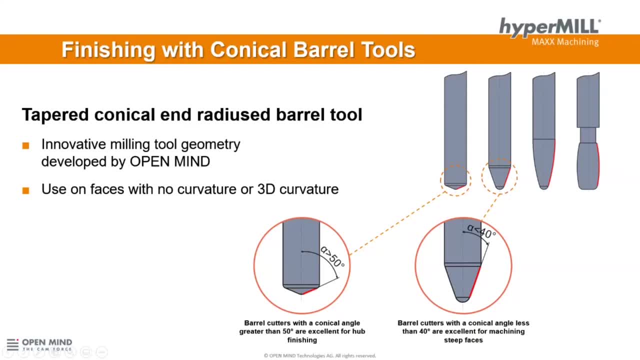 So this is where the tool is- is very effective and, as a taper, forces the tool to tilt, avoiding the collision between the parts and tool holder, And the ball nose allows us to use a same tool to finish areas such as small radiuses in the corners of deep pockets that I mentioned. 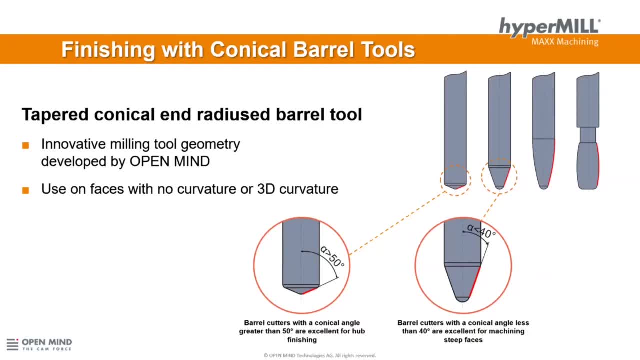 previously So because you're tilting the tool away from the part. this allows you to keep the tool length to a minimum and therefore tools are more rigid and less likely to produce torque chatter. So the potential gains can only be achieved if the cam system has the necessary 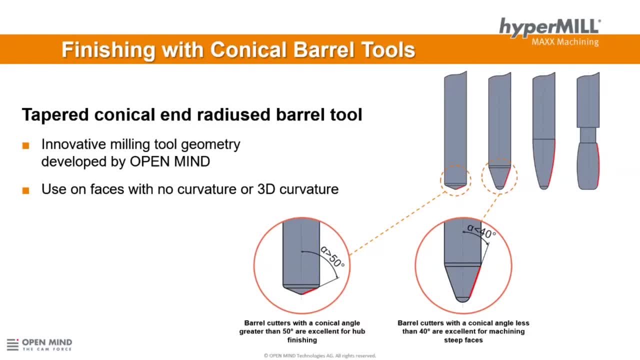 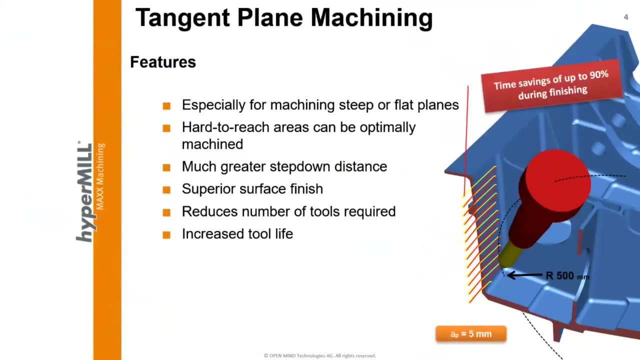 cycles, as Andy has just mentioned. So to utilize these types of tools within HyperMill, there are dedicated cycles that have been developed especially for use with conical barrel tools, and I'll explain what these are. So the first one is tangent plane machining for planar surfaces. 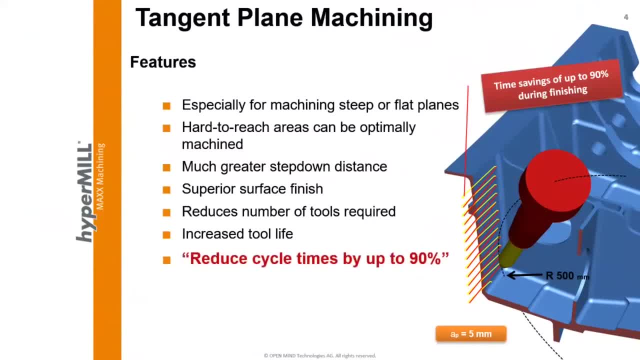 and it's extremely useful when machining deep pockets and hard to reach areas using conical barrel tools. Now, typically to machine a deep pocket such as this one here, a ball nose tool would have to be used with a head tilted over to avoid the collision with a tool holder. but you would only be stepping down probably what 0.2 of a millimeter for. 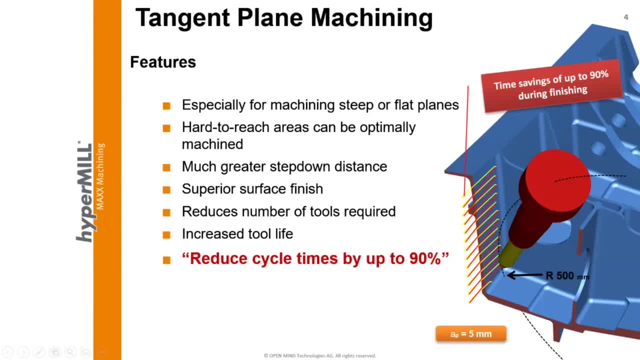 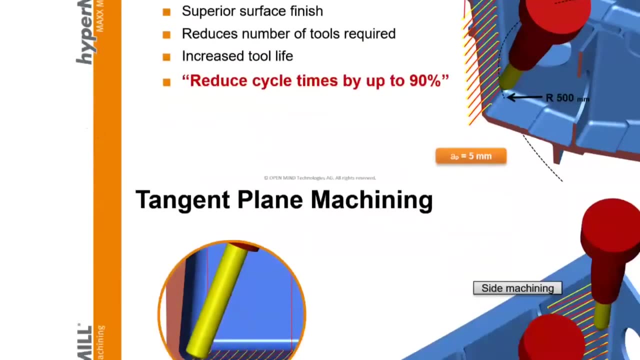 instance, so the machining times will be obviously much greater. However, with a combination of conical barrel tools and HyperMill tangent plane machine, you could be stepping down up to up to six millimeters, yet really still achieving a superior surface finish. Here's another example. 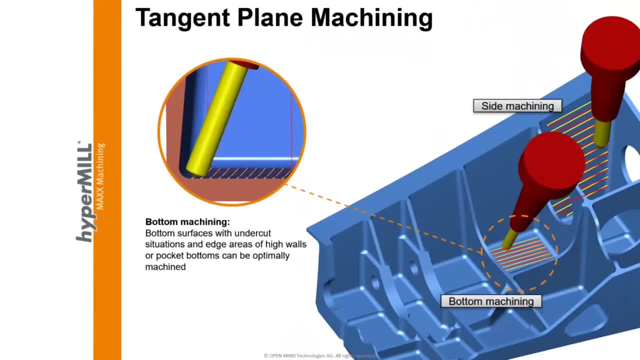 of a lens style conical barrel tool where the barrel radius is on the bottom of the tool, and these tools are useful when machining the bottom surface of very deep pockets. A conventional end mill couldn't be used in this instance because, due to the sheer depth of the 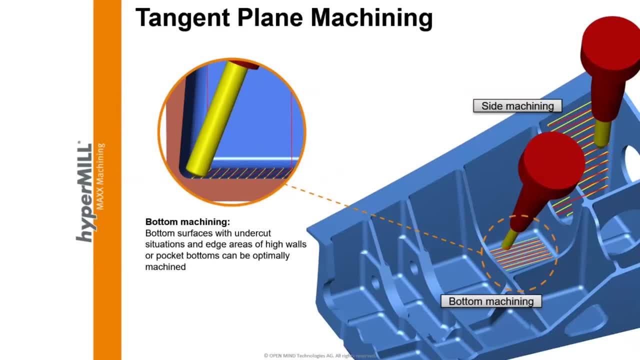 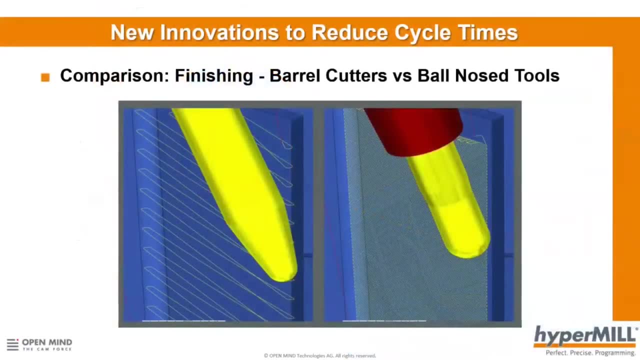 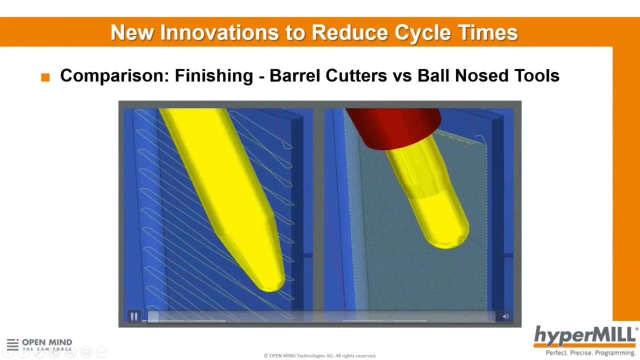 pocket. that would be. that would be impossible because the tool will be too long. So, again, the tangent plane machining cycle will be used for this face, this face also. So let's compare the machining of a planar surface using a ball nose tool And the 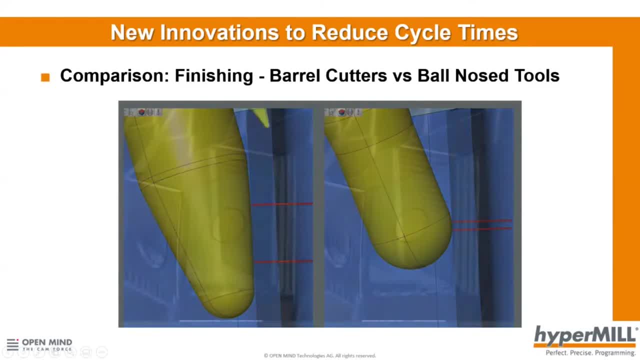 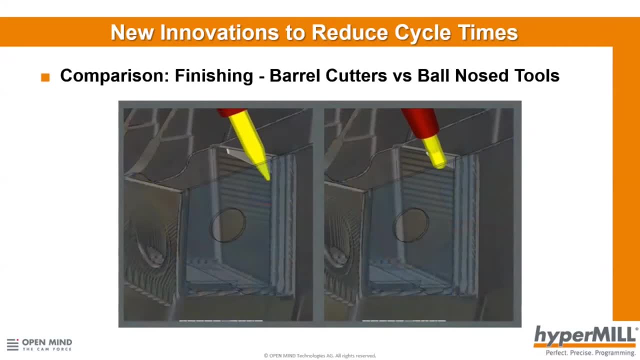 technology behind all of this is now, And to achieve this, We have a really high quality tool and we have done a wide range of technical analysis here at the company. I'm just going to give you a little time to get this off screen. 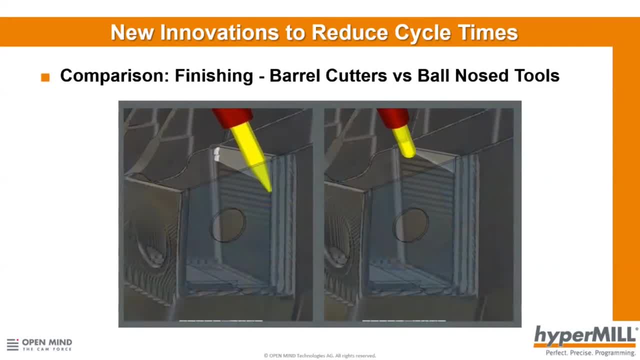 And the first thing that you notice is the turning on. the as a tool is traveling along the face. the head is built, being tilted simultaneously away from the surface, and this avoids the collision between the holder and apart and also reduces the excess material left in the corners. now, if i can stop the video at this point and just go back one moment, 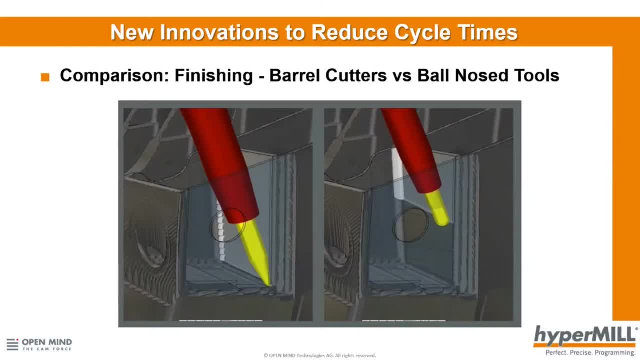 just slightly so the very fact that we're stepping down at six millimeters. this will leave a wedge of material in the corners, but within the same tangent machining cycle- and you can see the wedges here- within the same tangent machining cycle- there is an option to clean up the corners. 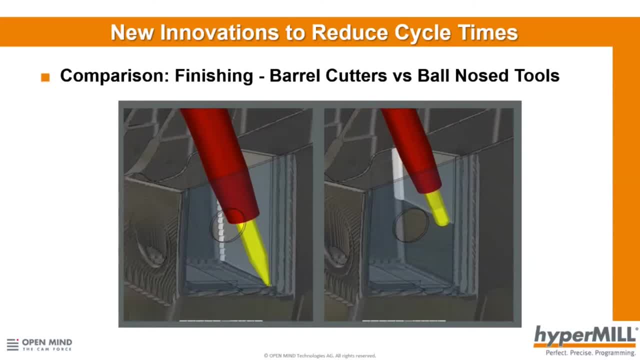 using a rest material style approach, using the baller of the tool, and i'll let that continue and you can see here. so, within same cycle, using exactly the same tool, almost two cycles combined into one, using both elements of the tool. so we conclude that this is a multi-functional tool and cam. 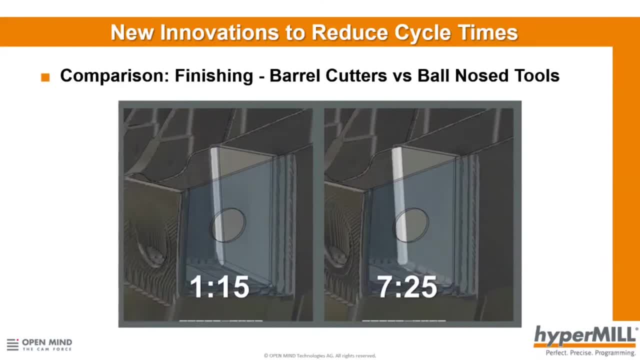 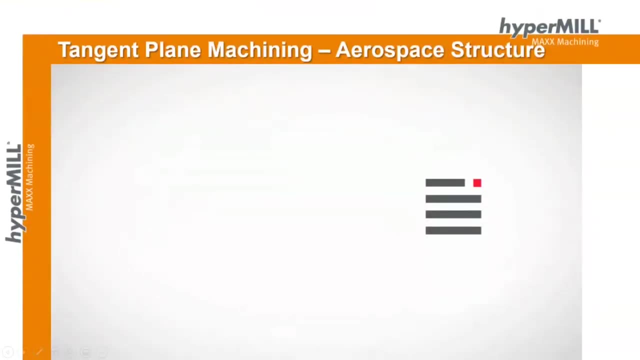 cycle to utilize the whole tool and reduce the need for additional tooling to be used. and obviously the time comparison says for itself: it's much, much quicker. okay, so here's the same cycle and tooling, but it's it's. we're actually machining an aerospace. 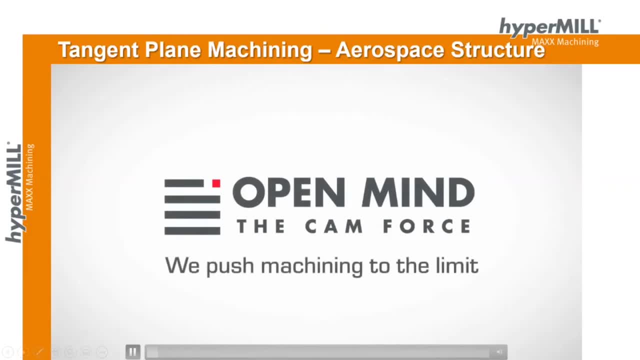 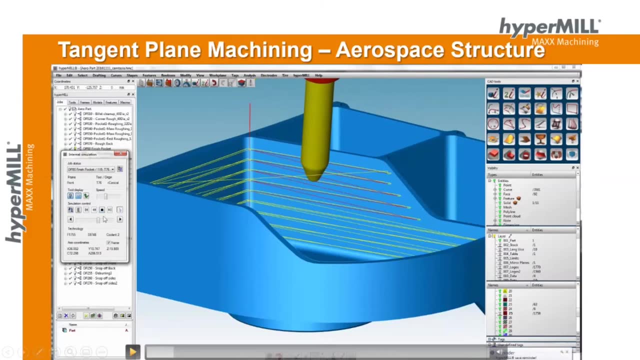 part now. i'm going to stop the video at this point once again, because you may notice that the head is fixed at the same angle when machining this area here. as it's, this edge of the pocket is open-ended, so hypermill is only moving ahead when necessary. 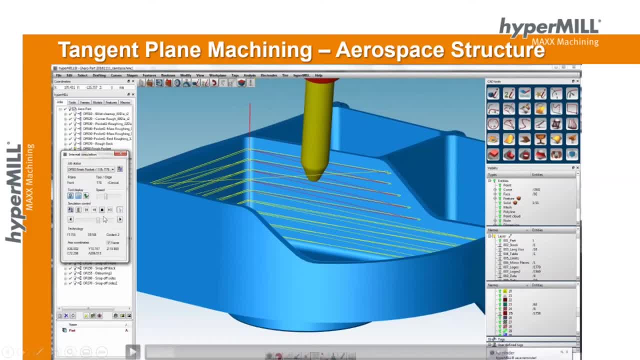 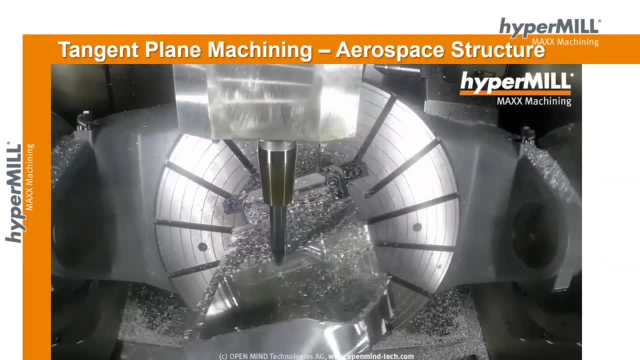 to avoid unnecessary axis movements, and you'll see that if i play the video, so it's fixing the head. no need to move the head. and now, only when it's the pocket is contained, does it then switch to a simultaneous five axis motion, and this is a completely automatic process. 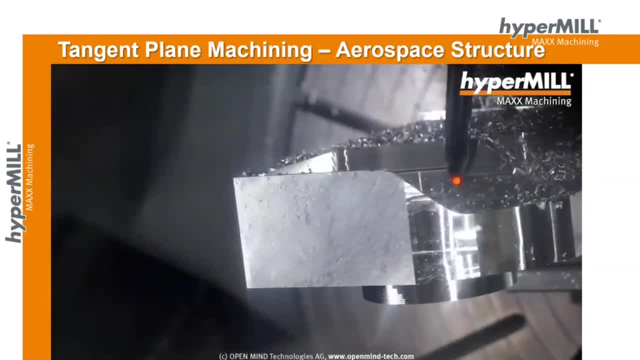 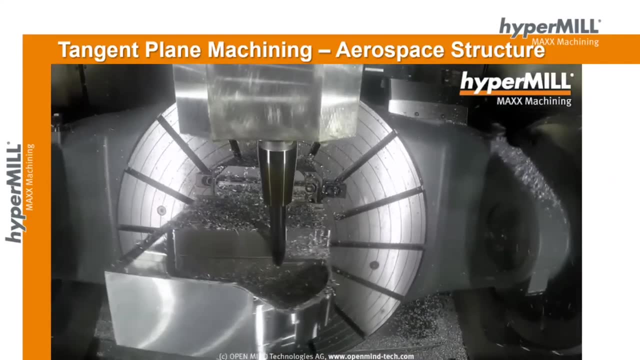 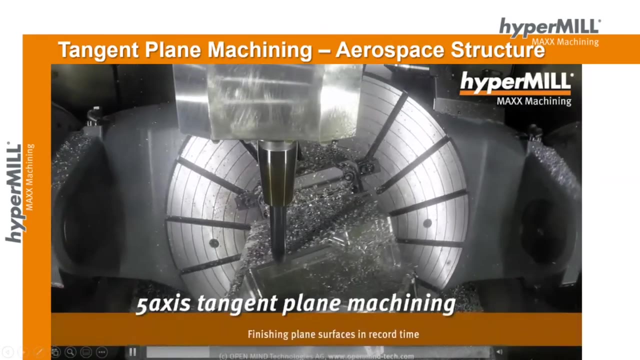 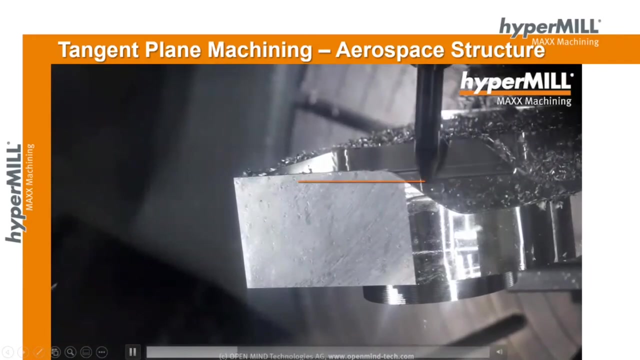 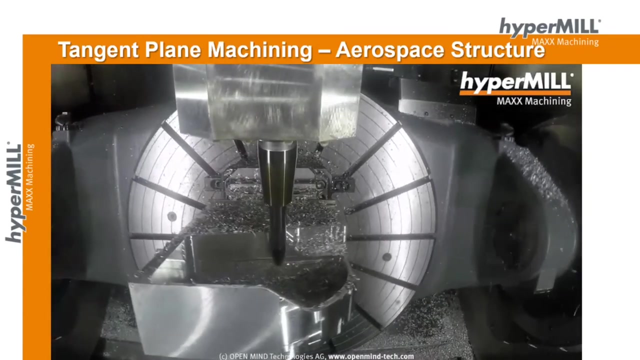 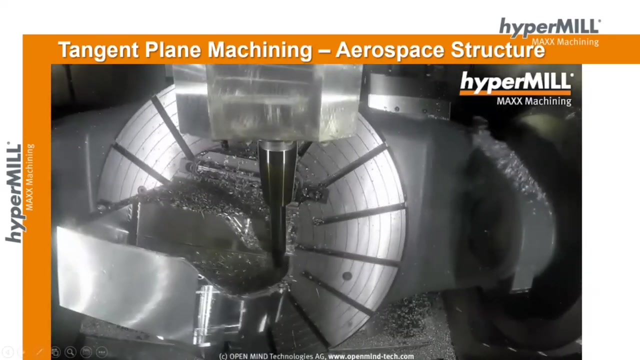 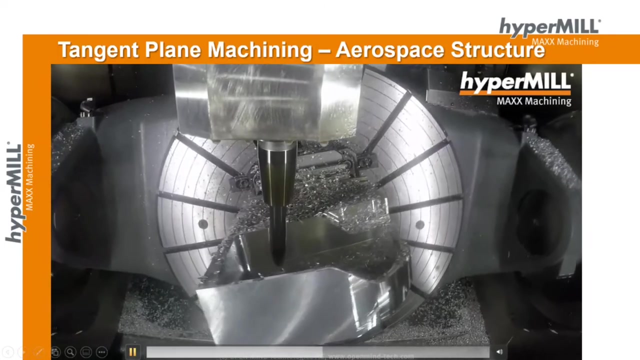 so here you can see it's fixed ahead. no need for excessive movement at this stage, only when it needs to, when it's it's within a contained pocket. now does it switch to the simultaneous movement. whoops, it's gone back again. okay, there we go. once again. it's fixed head position within a contained pocket. it now switches. 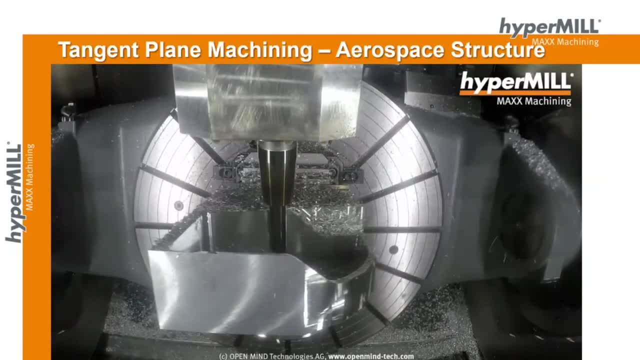 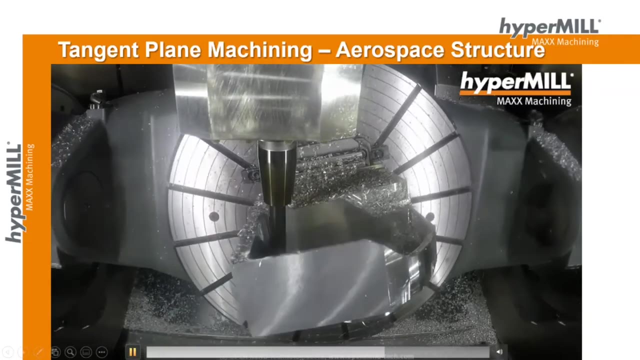 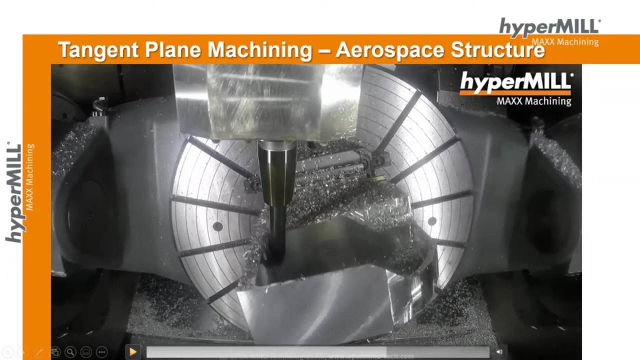 to a simultaneous movement completely automatic cycle. it's probably one of the easiest ones within hyper million fact to to program because it's simply a process of selecting the surface and hitting go, let it continue, and this is the portion it once more. this is where it flicks to the ball of the tool to pick out these wedges left. 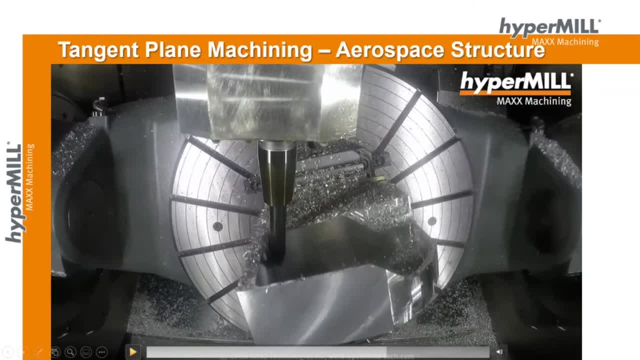 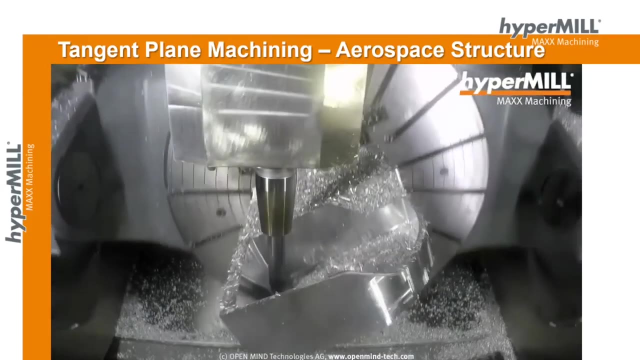 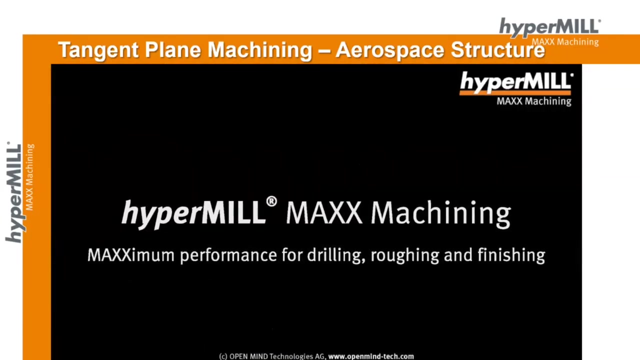 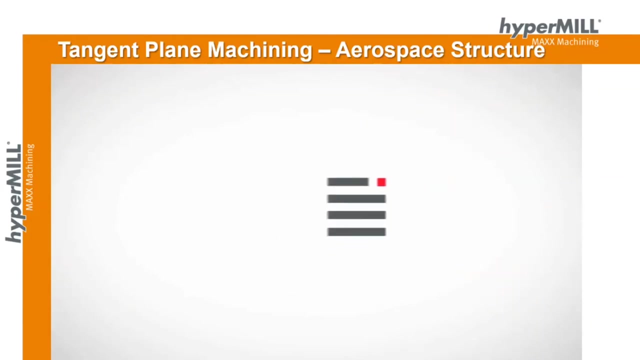 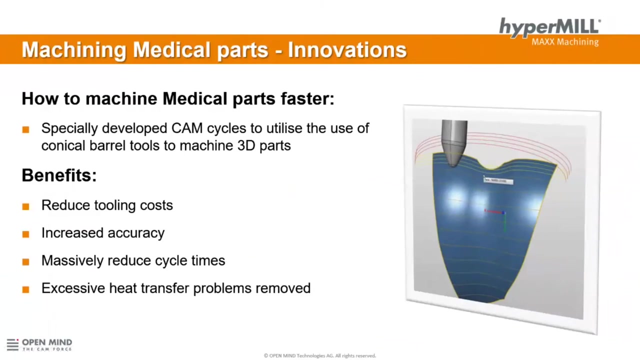 that the the body of the tool left in the corners and these are automatically removed in, as I mentioned, almost like a bounding or a rest material process: one tool to do the whole of that pocket. okay, so now let's move over and focus on where these tools and cam cycles can be. 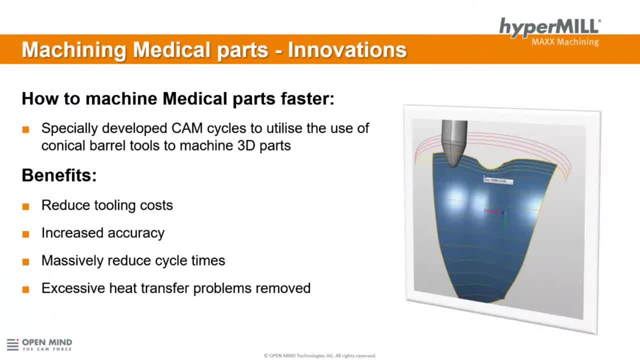 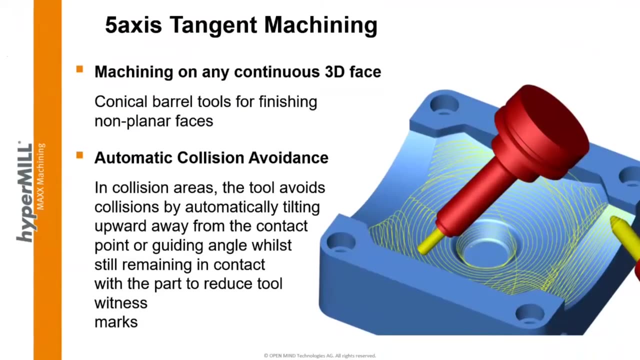 used to machine medical parts. now, in this instance we'll be looking at a femoral knee surface again. we can achieve a massive cycle time reduction and reduce tooling costs. I mean we really can increase the accuracy of the machining also. so the previous cycles that we that we used was called tangent. 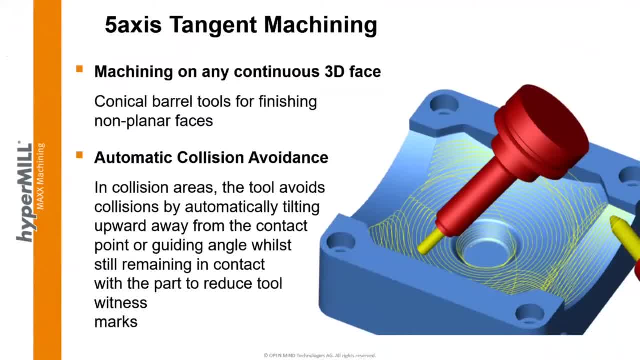 plane machining for planar surfaces, but now we were actually seeing a 3d face, a face, and this is where we use tangent machining, and these can be convex, concave, doubly curved surfaces and we have a cycle called simply, as I mentioned, tangent machining for 3D faces. 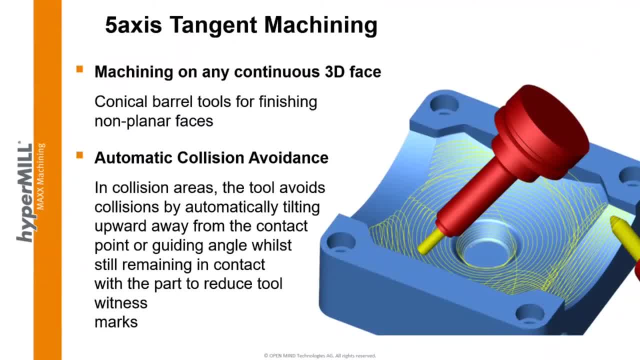 Now similar to the tangent plane cycle in collision areas, where the tool is automatically tilting upwards away from the contact point while still remaining in the contact with the part to reduce witness marks. Obviously, the more we retract, the more we re-enter the part. this will leave unwanted dwell marks, for example. 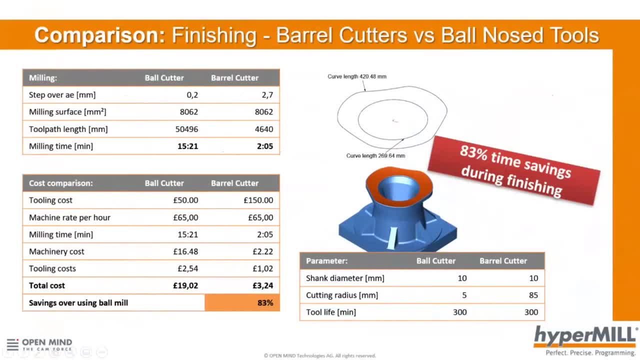 So if we look at this area of the part that was machined conventionally using a bullnose tool and then again with hypermil tangent machining using a conical barrel tool, when we weigh up the cost of the tool, The machine rate per hour against the total machining cost, although the cost of the tool 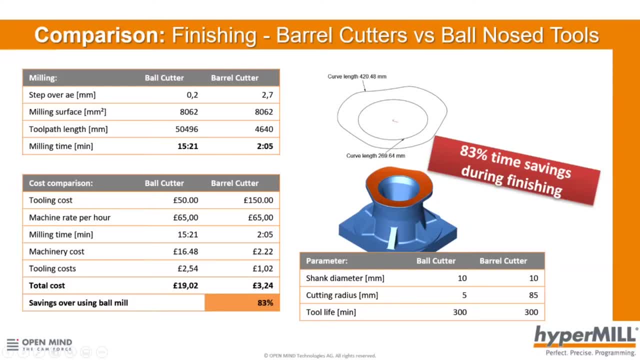 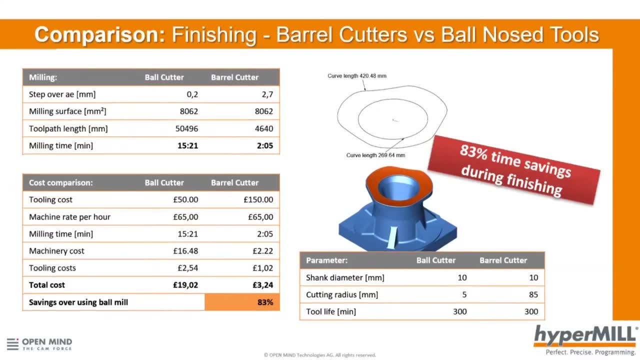 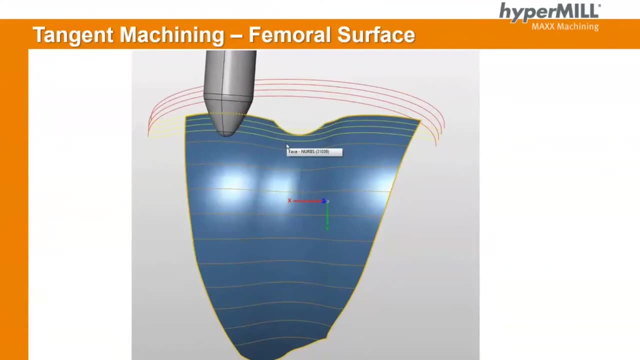 the barrel tool is higher. the total saving is actually 83%. so I think you'll find that's quite staggering. So it's plain to see that conical, the combination of conical barrel tools and hypermil max machining cycle is much quicker than conventional methods of machining. 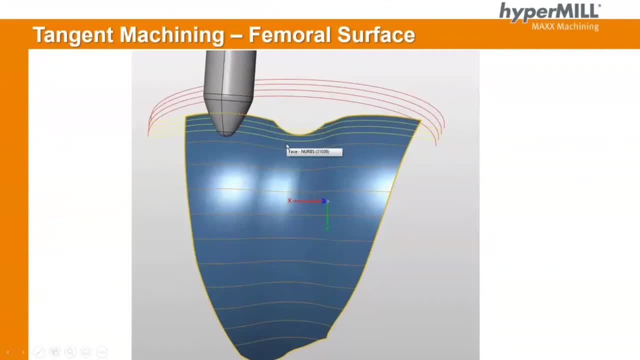 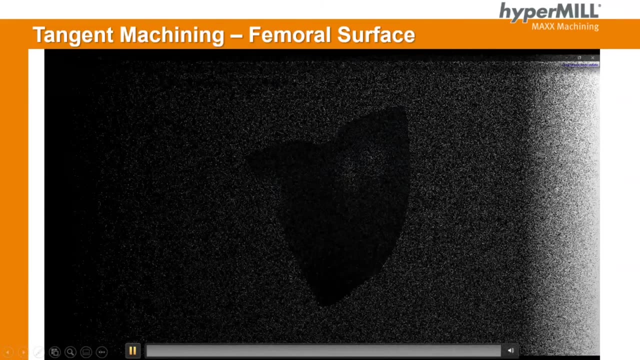 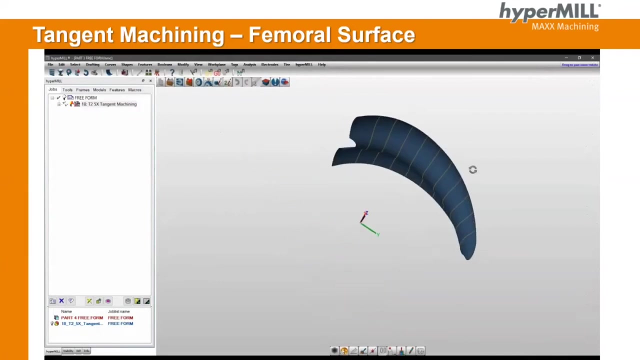 But let's see how we can put this into practice. practice to program this femoral surface. We're not limited to what type of surface we can machine. okay, this is a complete, you know, organic shape, as as many cases in the medical industry, and here I've actually included spindle geometry. 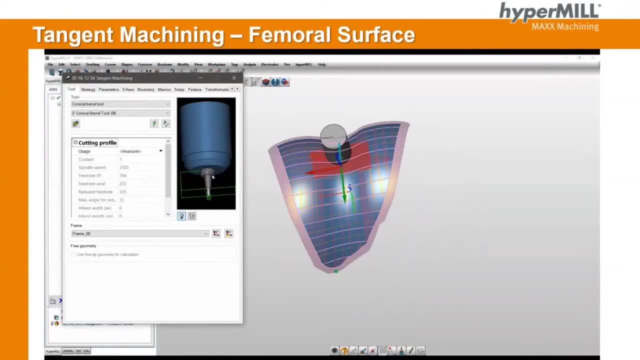 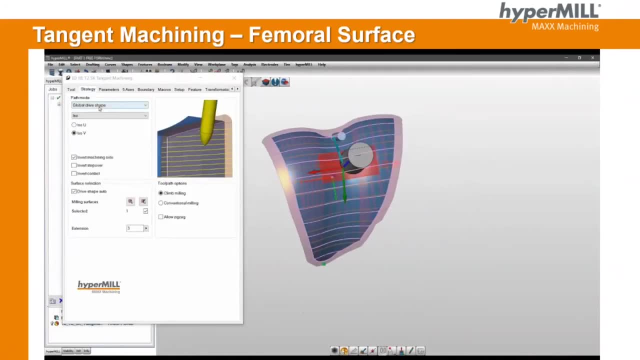 It's a noise reduction machine. The noise part of our software is that you can actually calculate and check against the spindle from calculation as well. you don't have to wait until simulation. So this is tangent machining and this is also a circle that has the capability for automatic surface extension, and it's quite nice for these areas. 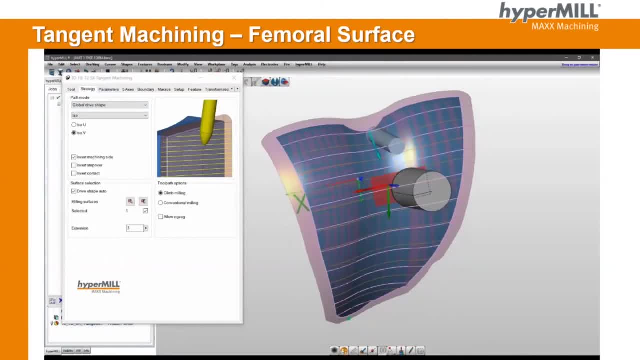 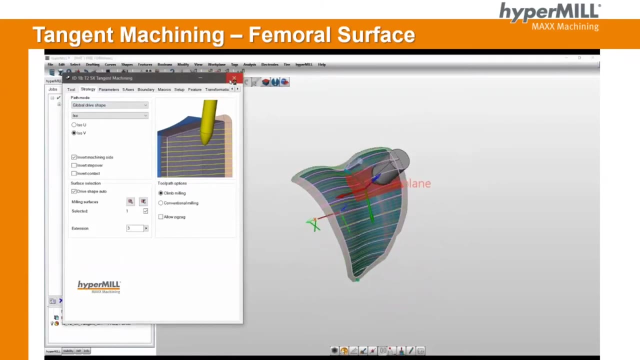 Okay, Certainly when you're doing freeform. So again, I've just picked the surface that I want to machine, I've just put it back into the Setter and that's it. that's kind of the actual free form that we're gonna get, and then we can get a real, real nice result going down here. 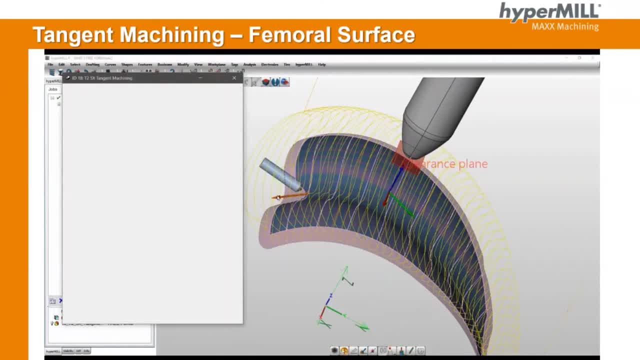 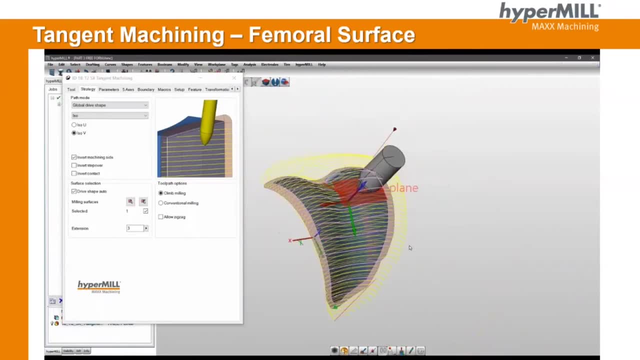 So what's not, what's nice about this tangent machining is So with with certain controls you get to, you get feedback on how you want the tool to Machine this surface, whether you want to go up down it, Which side of the surface you want to machine. 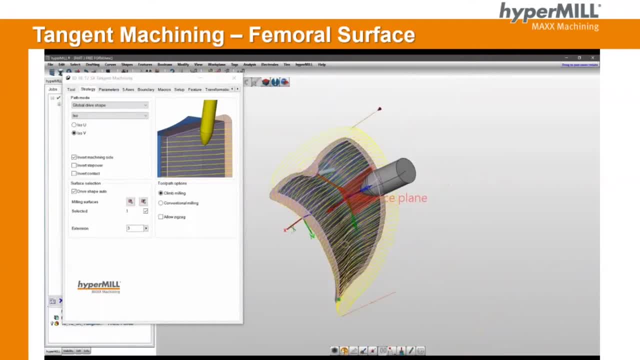 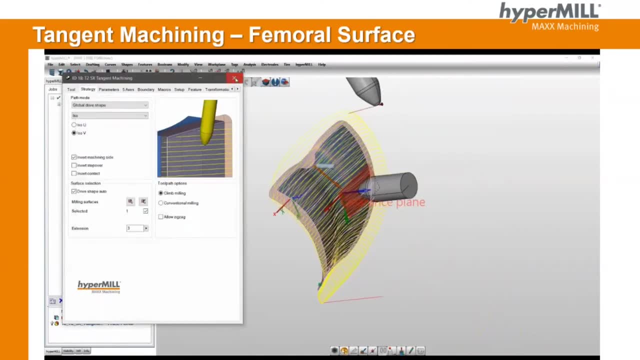 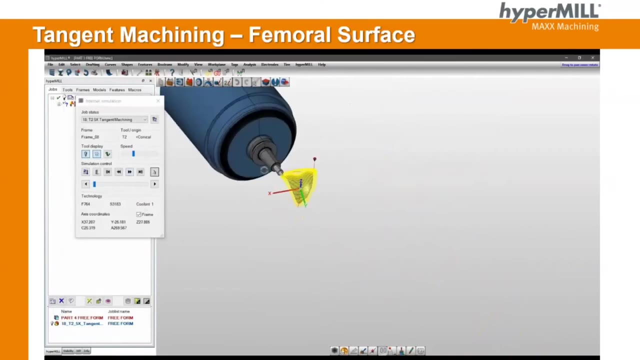 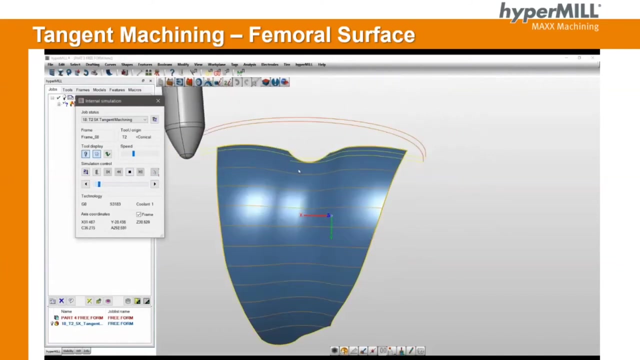 back as to as to what it's going to produce. now you can see this is a lovely, clean toolpath, actually. that's it's created. we'll just close the cycle for a second. okay, so we can see it tracking the surface. obviously, the surface extension did fill in the gap in a little bit, but you know, the less reach acts you have to. 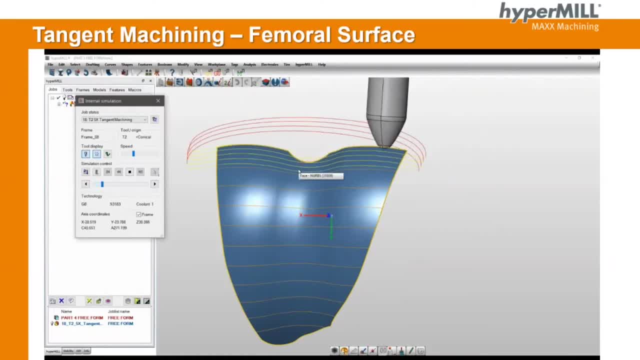 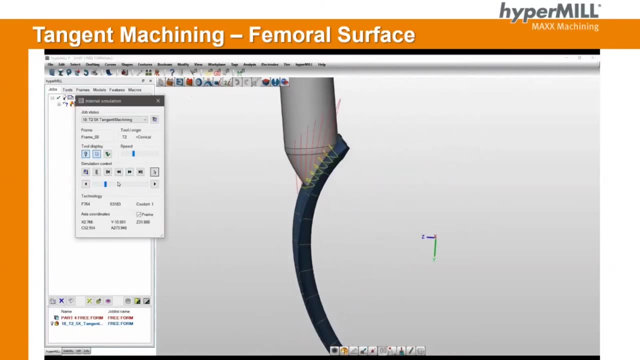 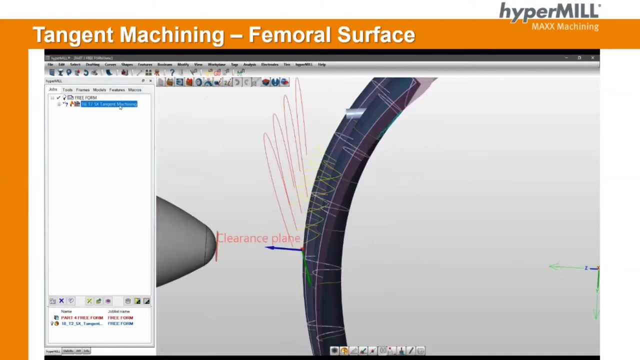 do off the part. let's read positions: the Bella. so that's where also it helps. you can see if I just turn the turn them model to the side a little bit, the contact at the moment I actually have set towards the tip of the tool. okay, so this is something we can actually manage inside hog mill is. 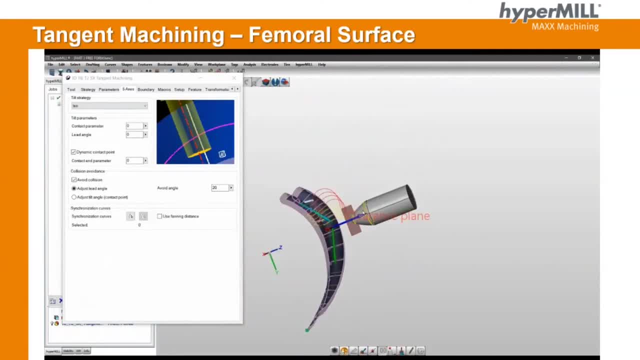 how much of that edge or what contact point on the circle segment are we using? now, when you're doing certainly hard materials, you could probably get quite heavy wear using the same point. you get notch wear and all the rest of it. what we have the capability to do is control the compact parameter, and it's 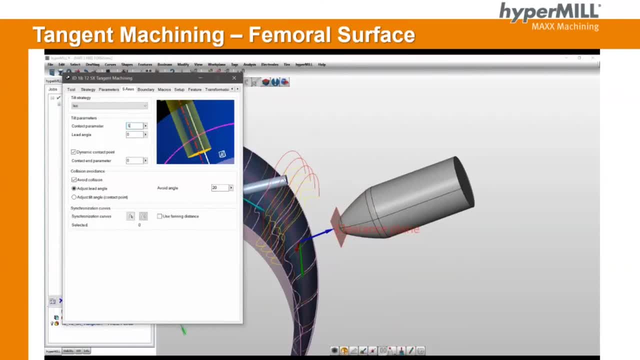 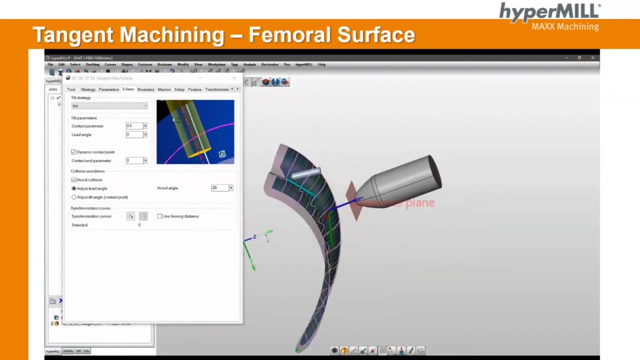 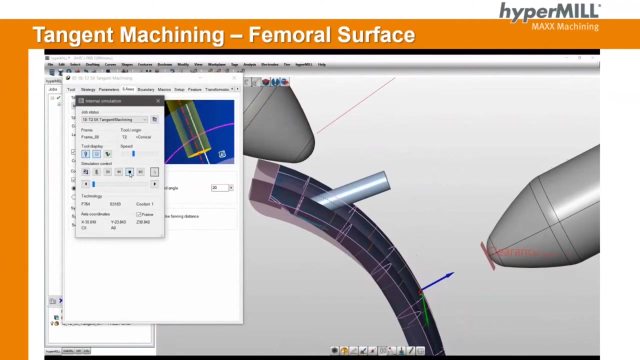 dynamic. so I could start at 0.5, which is halfway up the barrel, and I could end on zero. so I'm utilizing the full edge of that tool, or I could start at one and then utilize it. okay, so you should see now first cut. see, the contact point is now half way up the barrel for the cuts and it will. 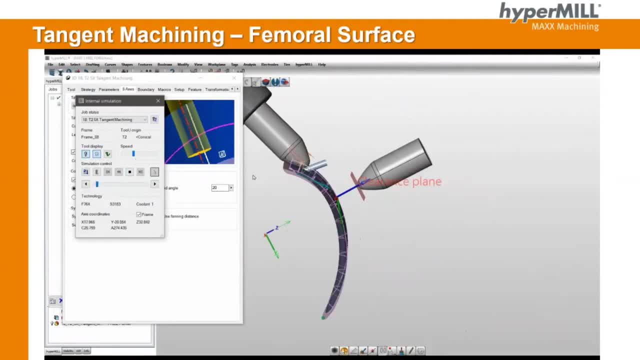 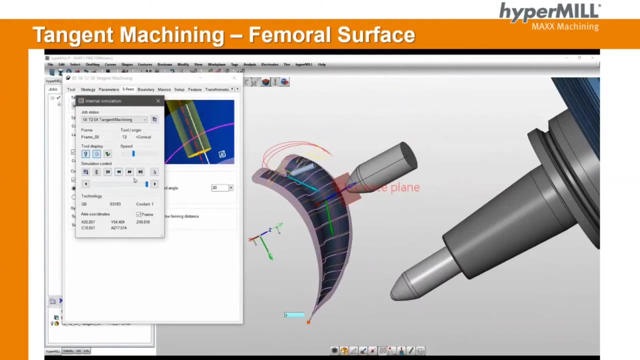 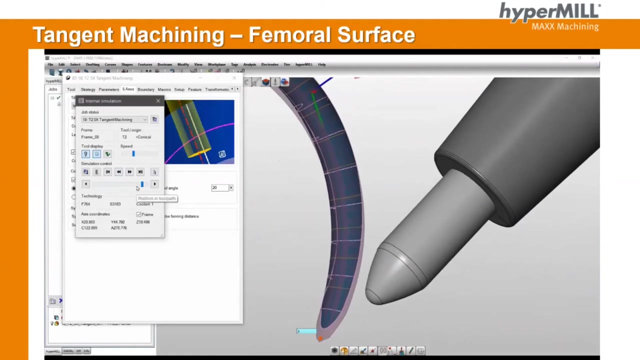 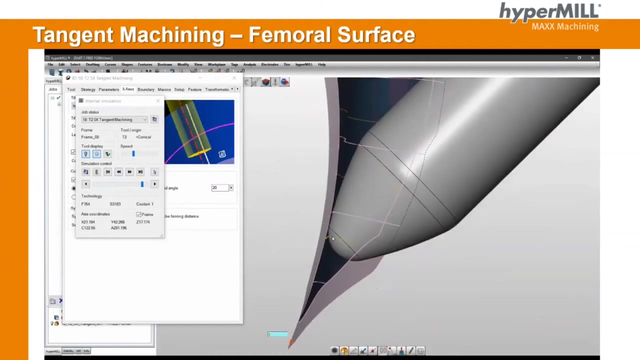 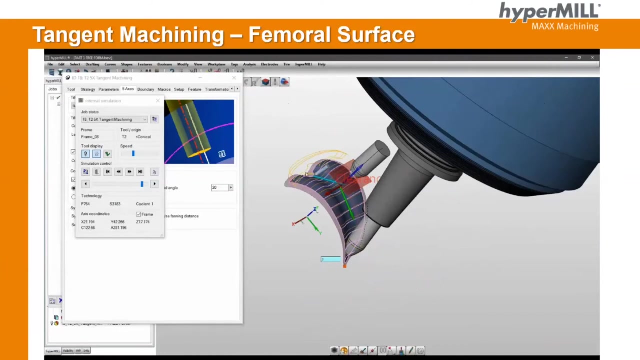 adapt and slowly change the contact point as it, the further it gets down the surface it falls to skip, maybe down to towards the end. I'll just rewind a little bit. you so now no longer utilizing half wear, all it's utilizing the tip, but that also, this control allows you to sort of eliminate the heavy first cut that you. 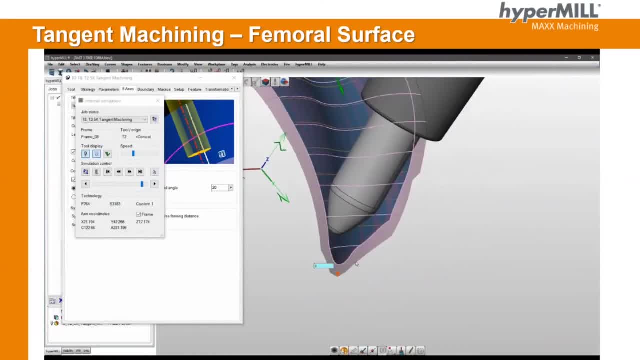 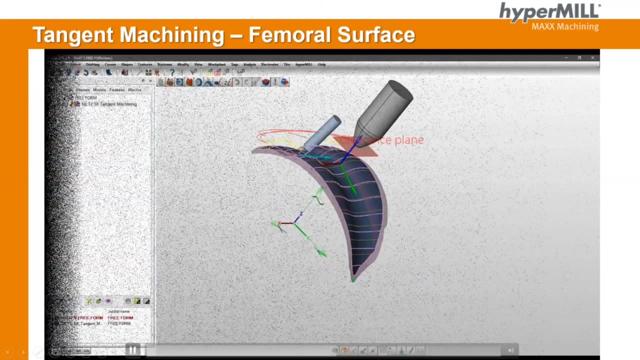 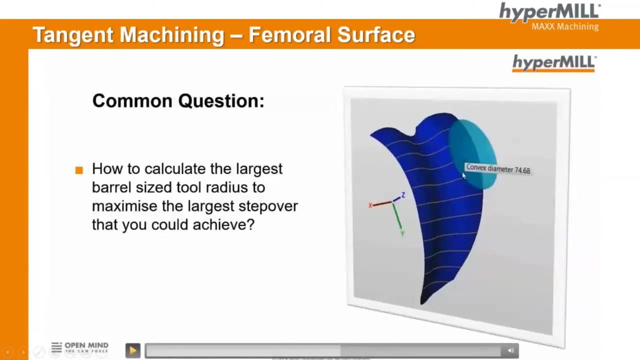 often get, and also the rest of material that will be left at the bottom of the surface. okay, by tilting the tool forward and utilizing closer to the tip, you get closer to the form and you don't leave the wedge of material. okay, so, yeah, I mean to have that level of control where you can vary the, the. 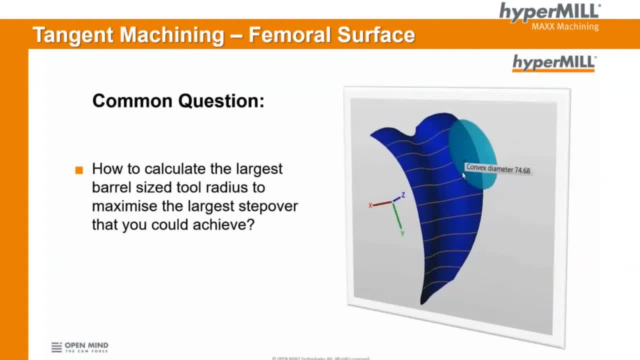 contact point you know, and gradually balance the wear of on that tool is really quite a innovative and unique feature, I believe. so keeping tool wear to an absolute minimum and having full, complete control over the contact point of that tool. now one of the common questions it's is, as this is a 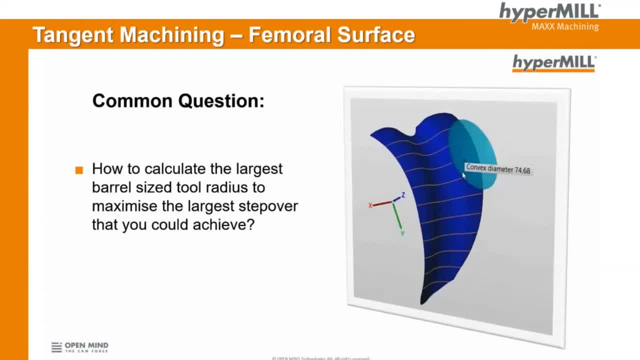 completely organic 3d surface or 3d model or shape. although many tooling providers provide off-the-shelf conical barrel tools, it's quite common that we need to use custom tools, and companies such as hard metal can provide both standard and custom tools. but how do we? 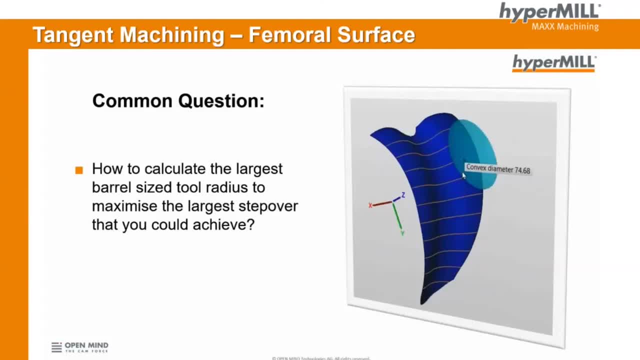 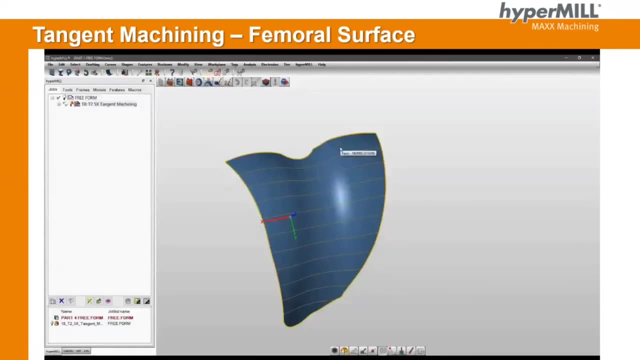 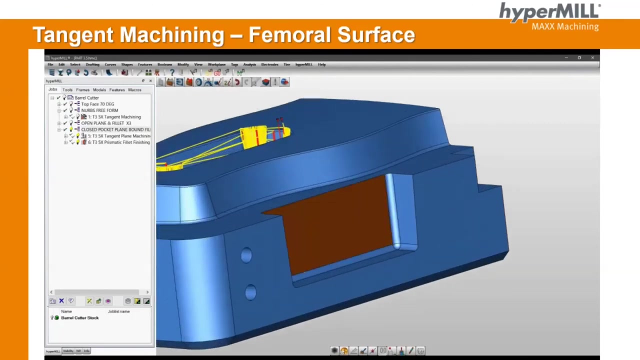 know what the geometry of the of the custom tool will need to be. so here goes okay. so the most common case of having or choosing your barrel radius size comes down to the geometry that you're machining. now, when you're machining flat planes, okay, you go as large as possible in here to maximize your step down, okay. 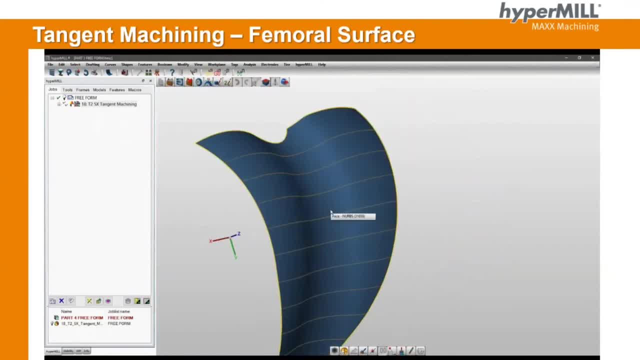 but with freeform geometry, it all depends on, first of all, surface finish requirements, whether these surfaces are being worked afterwards- I know, in this instance, this- these surfaces actually finished, so they're only after sort of a finishing operation. that gets you to within sort of point one, point two of the surface as quick as possible. and that's where, where 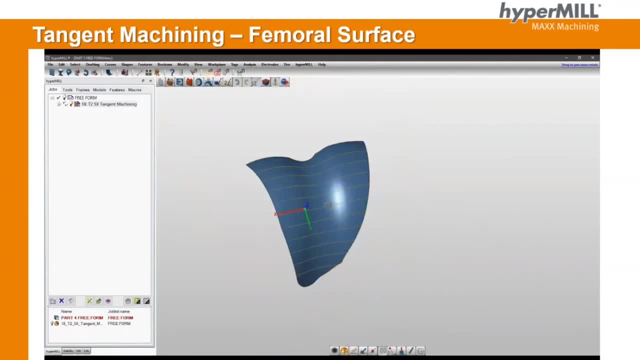 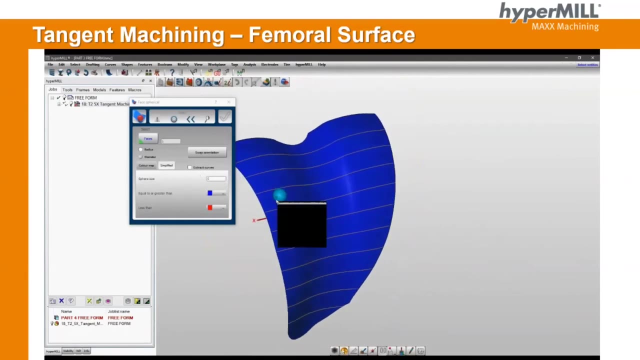 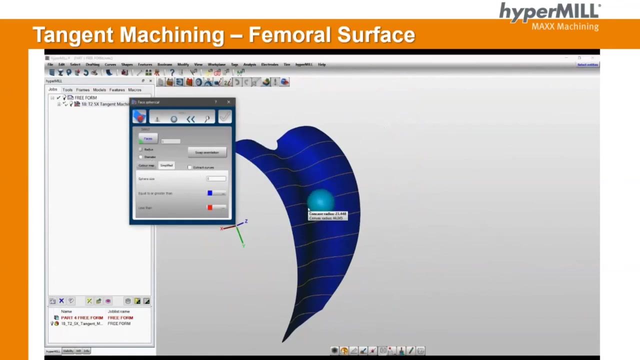 barrel tools have come in on this surface. to select my barrel tool size, I actually look at some of our analysis tools and we've got the tool here called face spherical. so for this surface you place spherical places, a ball or radius on the surface and by increasing or decreasing the sphere size you can start. 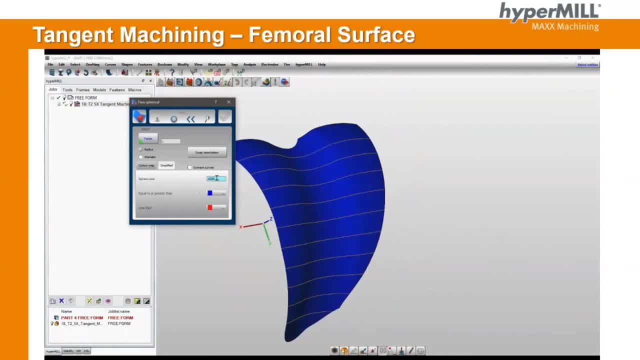 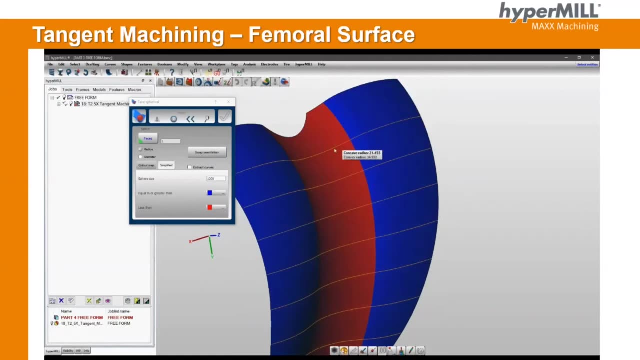 to see failure. so it's quite often common to get a barrel mill with a thousand radius. so I'll type in sphere size on radius mode- a thousand. I can see tracking over the surface instantly red. I'm gonna struggle to get the tool tangentially in there for a nice roll around. so that to me is an indicator. 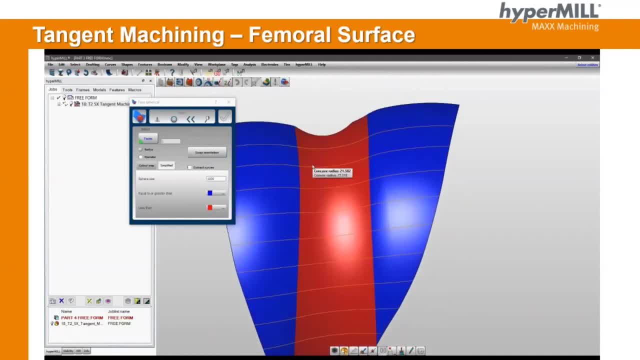 right, I need to start decreasing my barrel size. I'm not properly going to hit all of the surfaces. now, when you're looking at tangent machining again, you're using drive surfaces. it's collision checking against the surface. so as long as it's rolling over, you know it's, it's not going to gouge into the model, okay you. 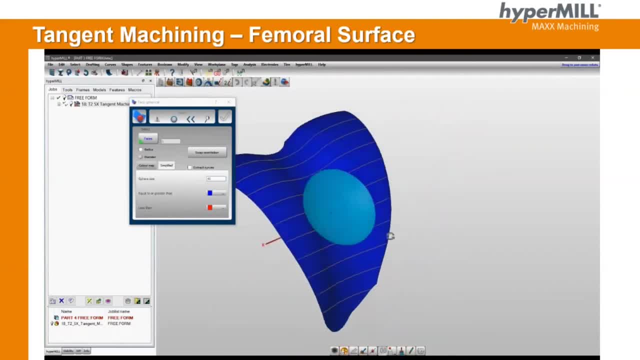 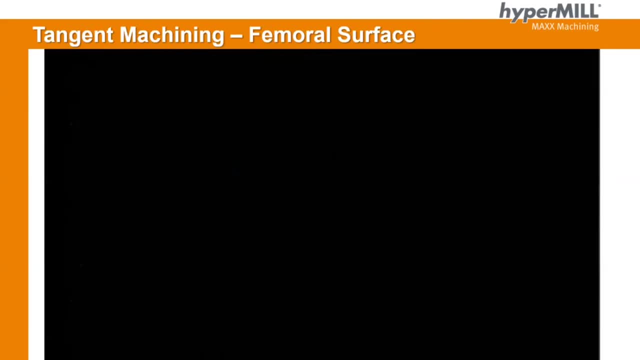 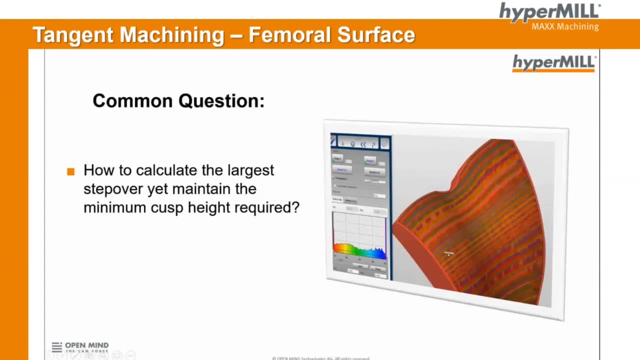 can see around the 40 mark on these areas. so this is this is a good tool to get a rough saw great. so another common question is: how do I know what step over to use to achieve the maximum cuts cusp height that would be allowed? obviously we can. 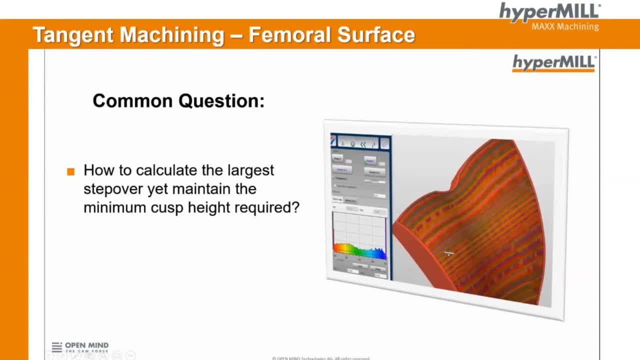 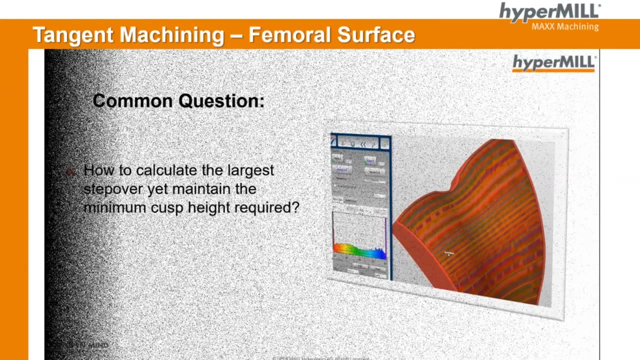 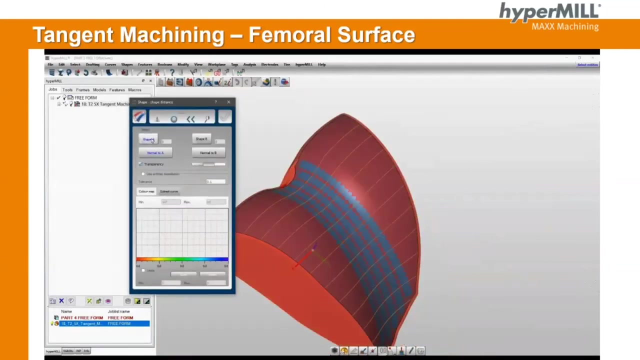 see that we can take much, much larger step overs when compared with with bullnose tools, but we still want to maintain that, that cusp height. so here we go. well, the one of the nice tools that we can use here is shape to shape distance. so shape shape distance means that one of the those different dimensions of the angle here is a었el, but it's made up by this line up, right by the line up, right down this line up by line up at the line up, line up at the 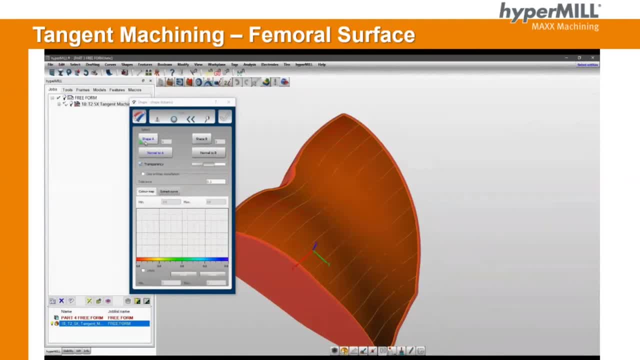 since I have my surface as one surface, shape a and shape B, I can use my stock model left over from the circle and, you know, with a little bit of tolerance in factor. so let me get to sort of 10 mark on tolerances. I can now get a really. 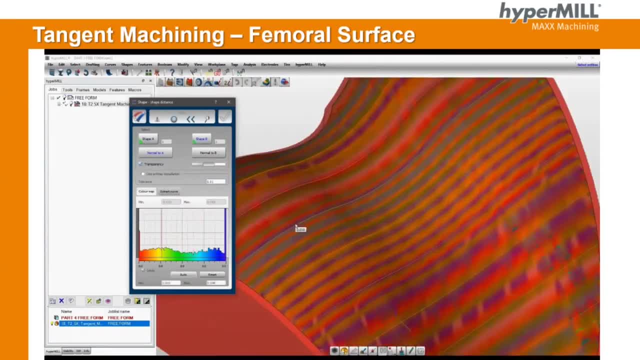 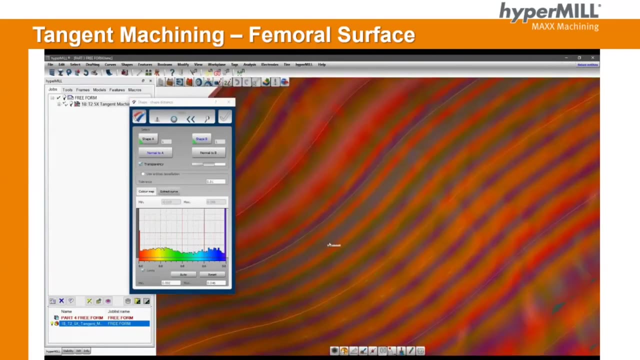 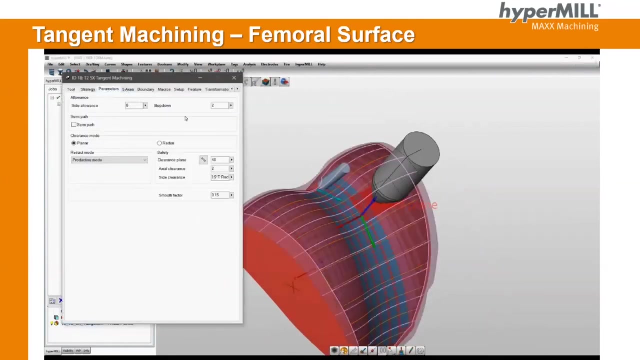 nice color map going of this area and feedback at cursor point as to my scallop pipe. okay, so I think with this, with this part, I've got 50 micron maximum I'll up left over from the barrel machining would absolutely you know, enough for this surface would be the work that's happening afterwards. but 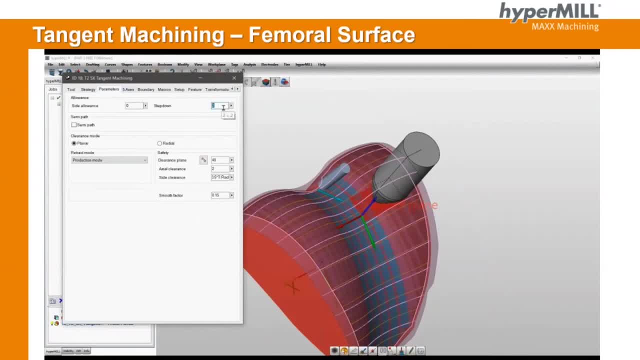 that figure is depending. now, okay, can I increase my step down by another milk and then the two mil. yeah, you, you just check in against what what your known parameters are. you just check in against what what your known parameters are and adjusting the tool size and barrel radius to suit to get the maximum. 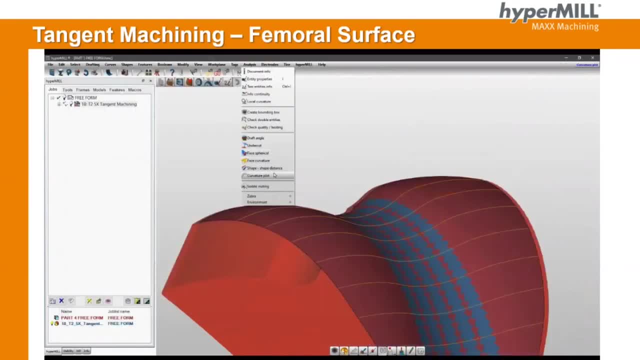 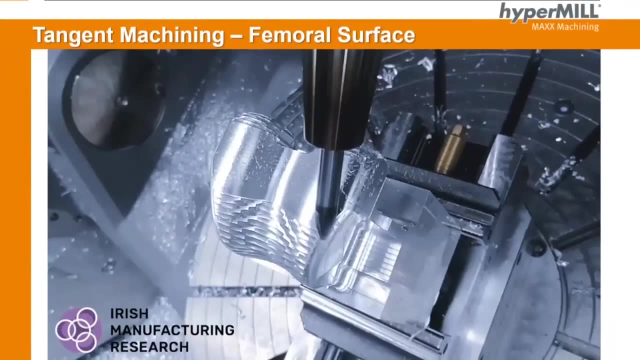 quickest result. so yeah, couple of tools that base, spherical shape, distance for checking the stock model afterwards. okay, super so, um. so the I'm are really very kindly cut this part on on their, at their facility, on their only c42, so that you can see the tool movement and see the surface finish you can achieve I'll. 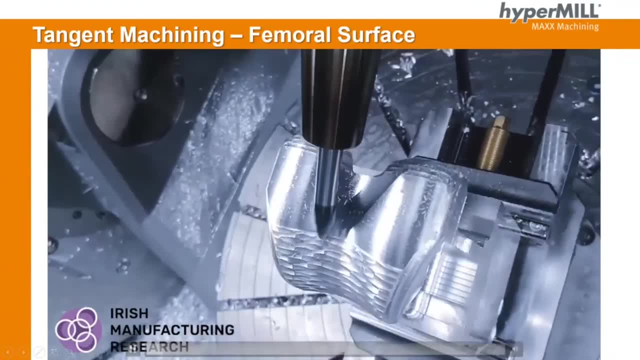 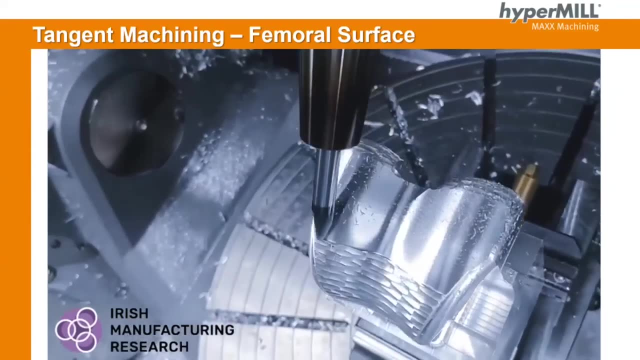 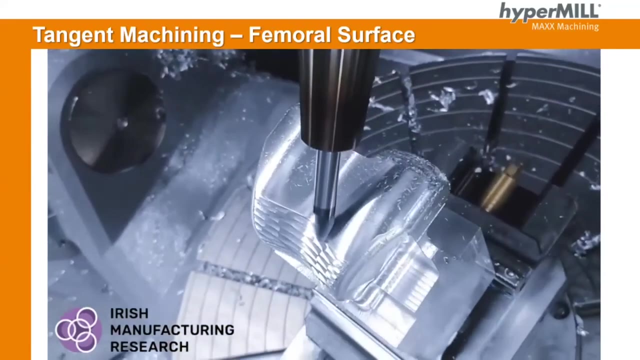 hope that you can agree that the results are all pretty good. the, the obviously hyper Miray's restricting the tool movement, that tool flying all over the place, it's, it's, it's a great surface finish well within their tolerance, that we need- and I must stress, though I- but this is only 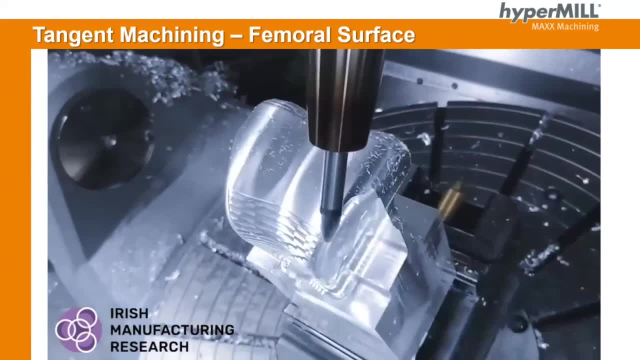 a concept part. so it was machine in our aluminium. so it was just to, Brady, give you an idea of how hard from is controlling the tool across that femoral surface. just to add to that, if epidemic sony used to point out that work within the patterns is to wear a menial, gave it 감사합니다めて. pom in the field was very goodness, Granny, from my own awning menial. quite a refuge. this was an Product 22анич het pew waste on our euhadipo. 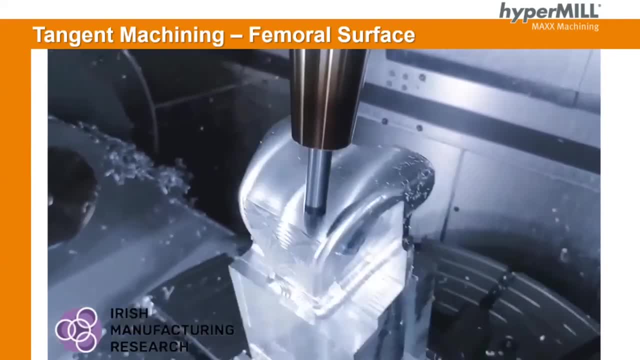 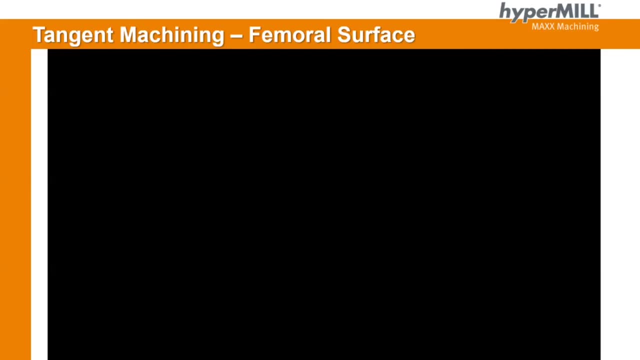 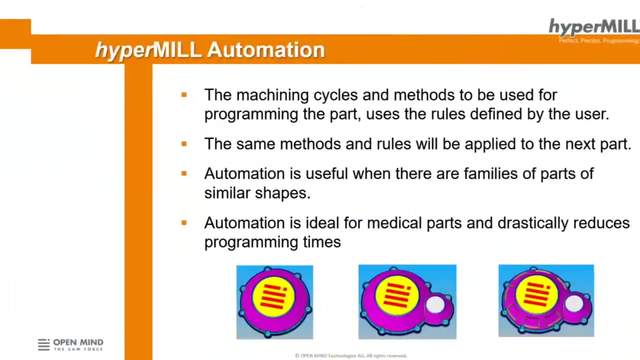 that femoral surface. just to add to that. if you don't mind, simon, just to point out that the tool that was actually used was a 10 millimeter iscar taper barrel tool. thanks, andy. okay, yeah, i'll flip to the next slide now. okay. last but not least, another real high level of growth. 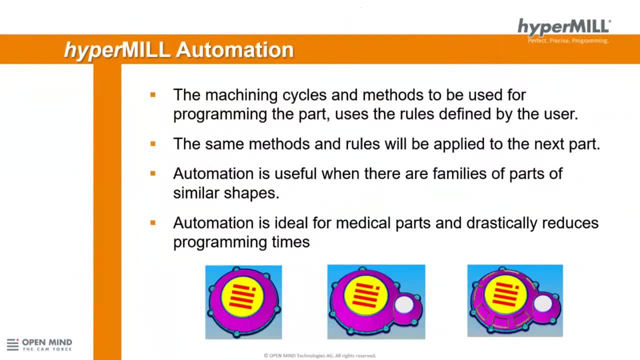 within the hypermil user base is is the use of hypermil automation now. it's designed to reduce programming times, especially for parts of the similar nature, or for parts, families of parts, as they may be called now. hypermil automation uses methods defined by the user and applies the same